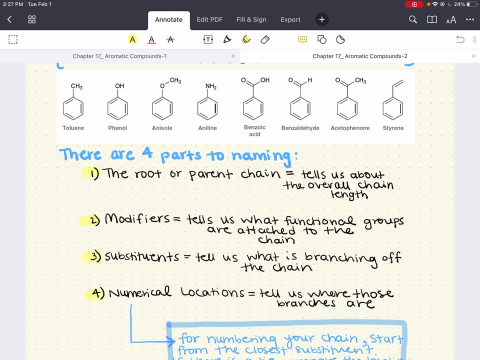 learned, Figuring out your parent chain, seeing if there are any modifiers, any functional groups that are attached to the chain that might change the name of the parent chain. what substituents are there and then where are they located? the numerical location of those substituents: 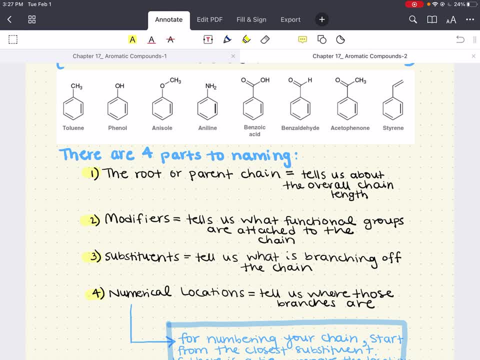 And, after we figure out each of these four parts, learning how to piece it together to determine the IUPAC name. Now, monosubstituted derivatives of benzene are named systematically, using benzene as the parent name And then listing substituents as a prefix. So a good example of this is: let's go ahead and 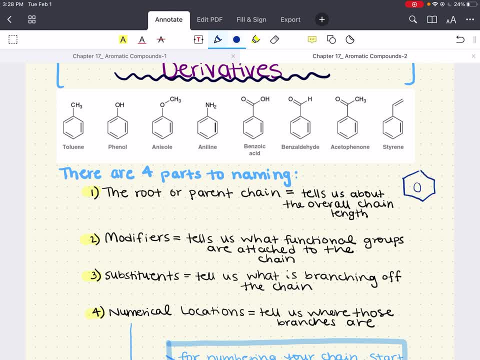 draw benzene. All right, this is benzene. If benzene had a substituent that was, say, chlorine, then the way we would name this would be chlorobenzene. All right, if the substituent that was here was a nitro group, then we would name this nitrobenzene. If it was. 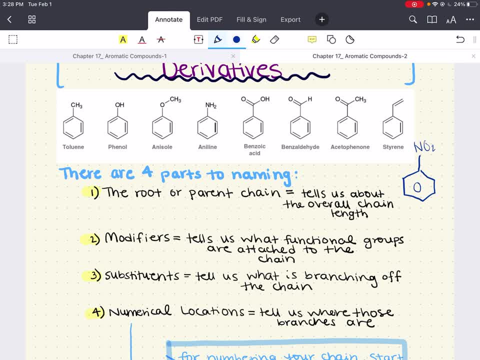 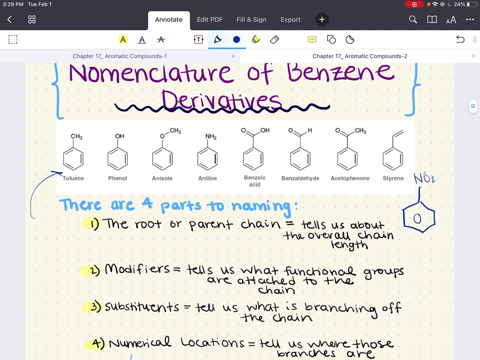 bromine, we would name it bromobenzene. Now the following: here are some monosubstituted aromatic compounds that actually have common names accepted by IUPAC. So, for example, let's distinguish this IUPAC and common name idea right. The liquid that you use to remove your nail polish is known. 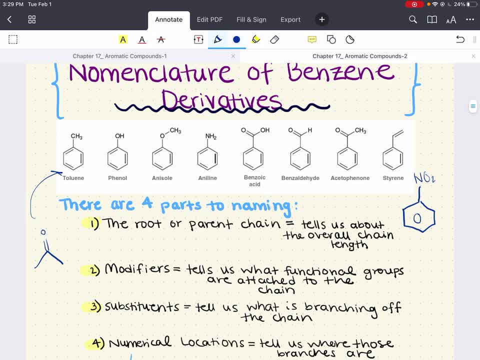 with its IUPAC name as 2-propanone. All right, it has a common name that you know it of as acetone. So here what we have is a list of monosubstituted aromatic compounds that actually have common names. 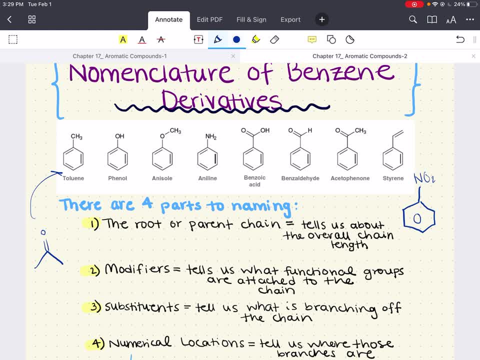 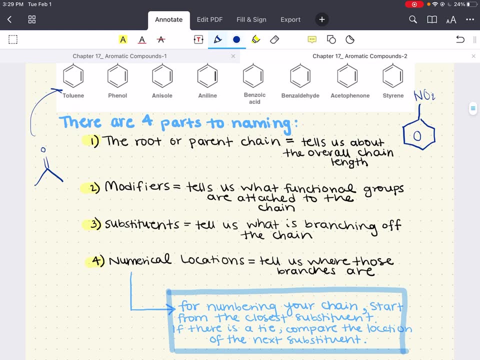 accepted by IUPAC. You must commit these common names to memory, as they will be used extensively throughout the remaining chapters for OCHEM 2, and they will pretty much only be used in the by their common name. Now, one thing to keep in mind, in addition to remembering the common name. 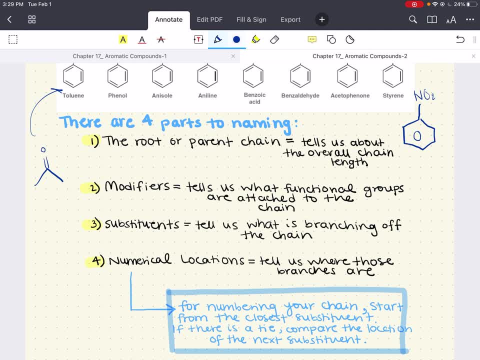 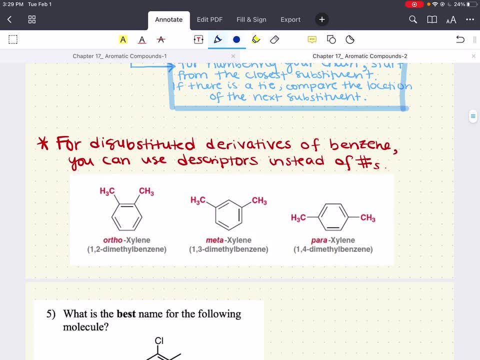 for these aromatic compounds is how to refer to disubstituted derivatives of benzenes. You can use descriptors instead of numbers, and we're going to go through this. For example, this is 1, 2-dimethylbenzene. We have our two substituents at the 1 and 2 position Now. 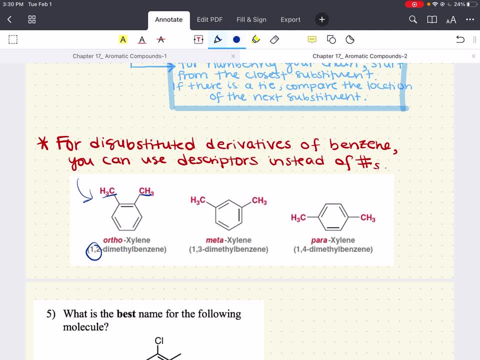 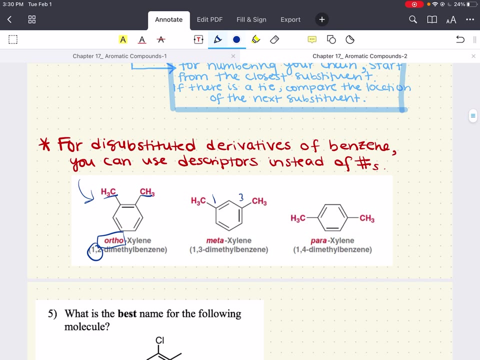 instead of using numbers, you can use a descriptor, and the descriptor for the 1, 2 numbering is ortho. All right, so we can refer to this as ortho for 1 and 2.. Now, what if our substituents are at the 1 and 3 position? All right, instead of using numbers. 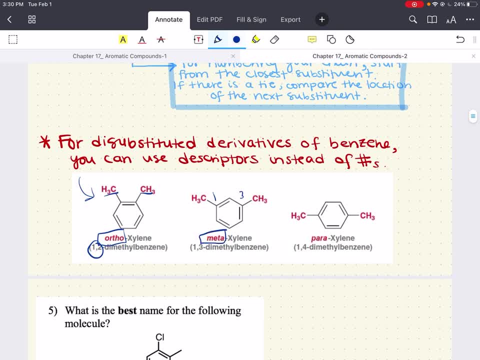 we can use the descriptor word meta for something like that, All right. and what about if our substituents are at 1 and 4?? All right, we can use, instead of the numbering, the descriptor term para for this. Now, what we really want to do is some practice. We're going to use the descriptor. 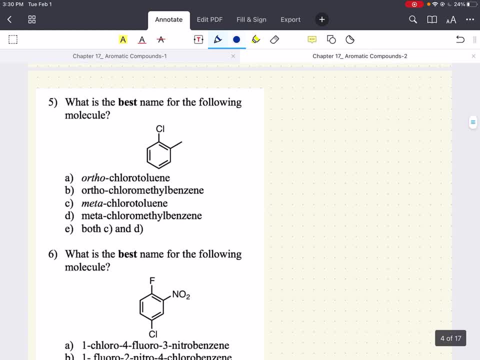 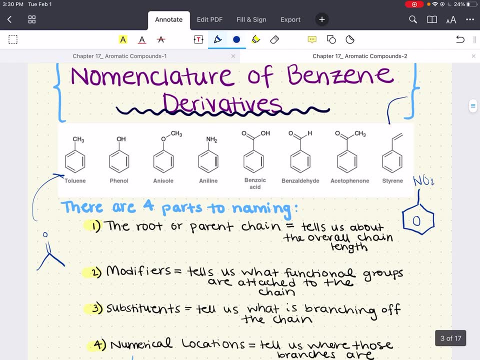 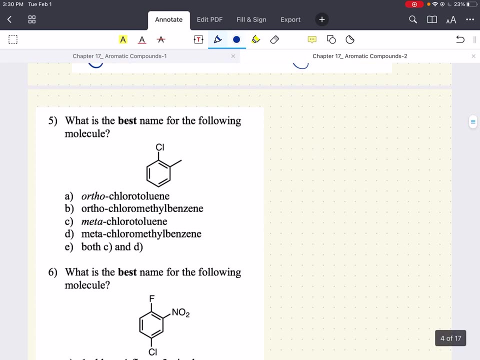 problems. just to understand this. and what we want to keep in mind is, if you are looking at a molecule that you can identify one of these benzene derivatives, then let that be the parent name for your molecule. All right, and let's see this with this example right here: What is the? 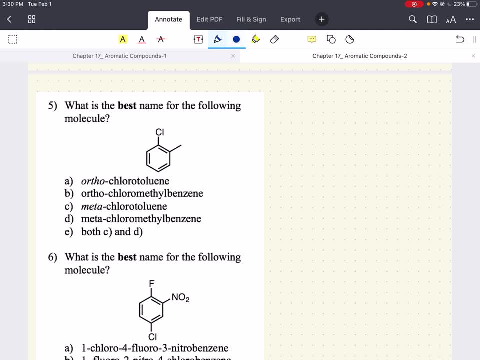 best name for the following molecule. If we look at this molecule, we can identify one of our benzene derivatives, and this is known as toluene. So what we can do is use toluene as our parent name, all right, and work from there. So we've identified our parent name. This is: 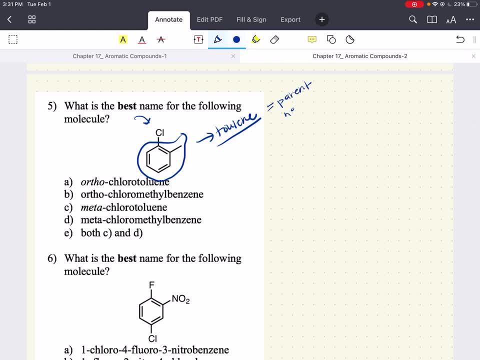 toluene. All right, does toluene have any substituents? And it does. It has a chloro group as a substituent. Fantastic. Now where are the chloro and the methyl group in reference to each other? right? This is one, two positions for the numbering here, And so, instead of numbers, 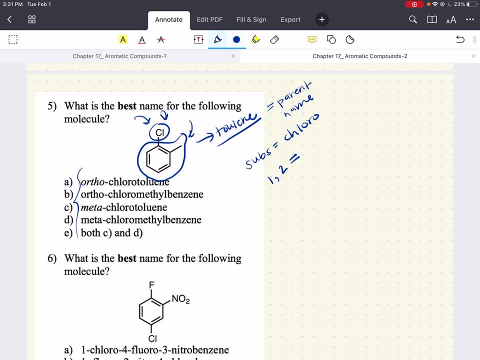 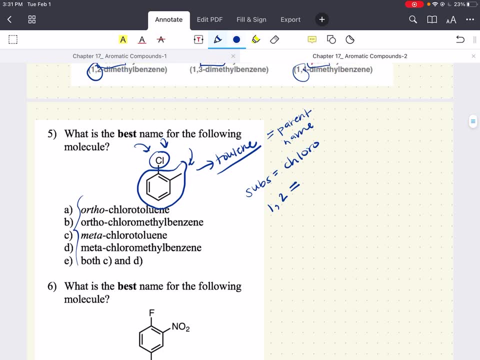 because if you look at the answer choices, they're clearly not using numbers here, So they're using descriptor words. So we want to fall back onto that to make sure we identify the correct answer choice. Well, the descriptor word that we can use for one two is ortho All. 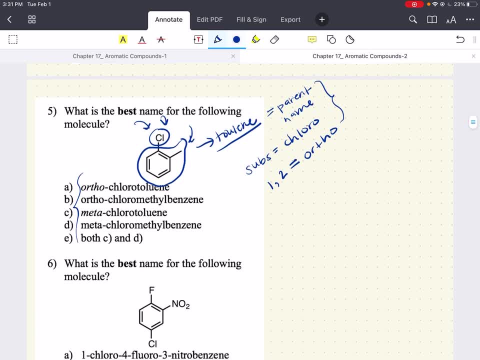 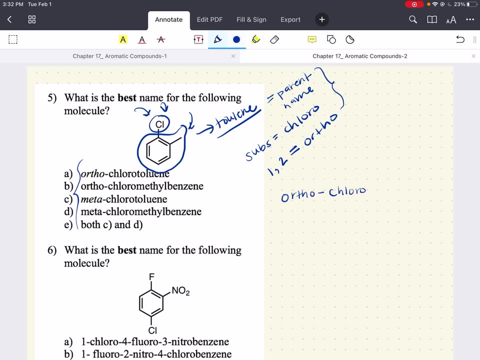 right, So now what we want to do is simply put these three pieces together. All right, remember substituents. We do our numbering And since that's the only substituent, we can go ahead and follow it immediately with the parent. 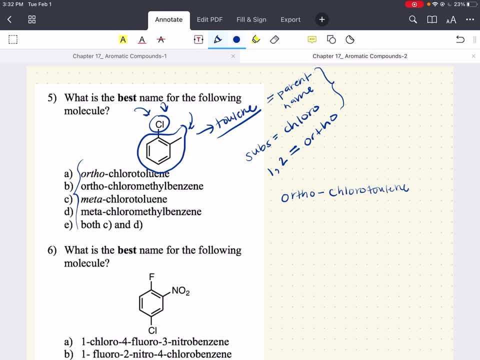 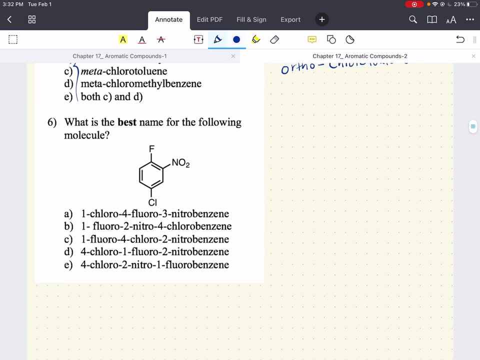 name. The name of this molecule is orthochlorotoluene. All right, that's the answer. choice A: Now let's do six. What is the best name for the following molecule? We have this molecule right here with a floral group, a nitro group and a chlorine group. All right, we don't. 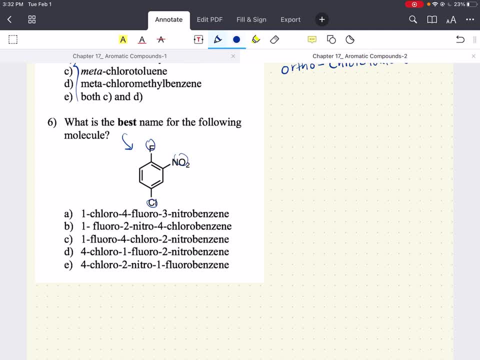 see any benzene. We don't see any chlorine. We don't see any chlorine. We don't see any chlorine. But we do see that we have substituents on a benzene ring, So we're simply going to use benzene here as our parent name. Now, on benzene, we have three substituents. They are fluoronitro. 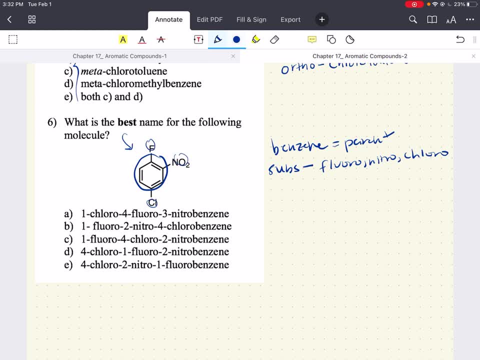 and chloro. All right, fantastic. Now we want to figure out the numbering for each of these. How do we want to number this? Well, if we start our numbering at the chloro group, one, two, our next number is three and then four. So we have substituents at one, three and four. However, 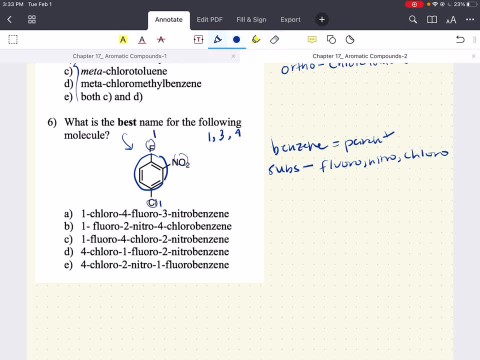 if we start our numbering on the fluoro group- one, two, three, four- then our numbering order will be: we have a substituent at one, at two and then four, And if you notice here you want substituents to have the lowest numbers possible. So we're going to start our numbering at fluoro. 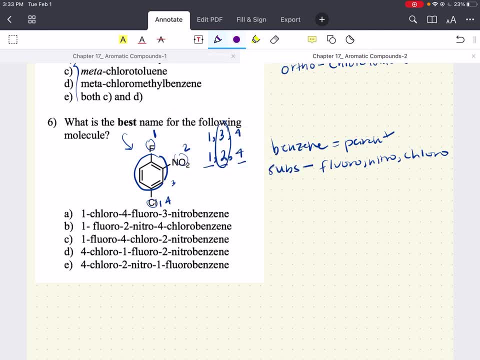 actually, And so that means that the fluoro gets the numbering one gets two and chloro gets four. We have all the pieces we need. Let's put it together, keeping in mind to do this in alphabetical order. All right, if you recall, from chapter four. 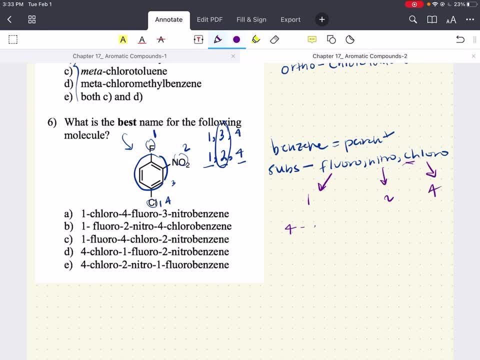 when we learned naming. that's very important. So C comes first. So four chloro- fantastic. Then we're going to do one fluoro and then two nitro, and then that's our last substituent. 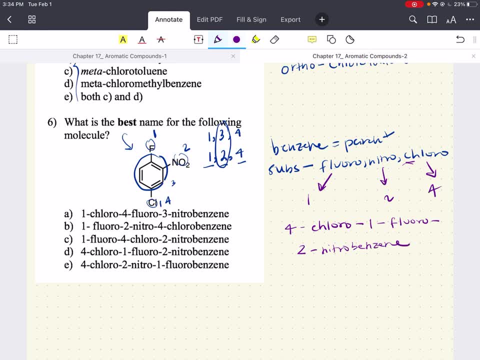 So we slap that parent name at the end here. So our name for this molecule is four chloro, one fluoro two: nitro benzene. All right, that's answer. choice D: Fantastic, So that's. 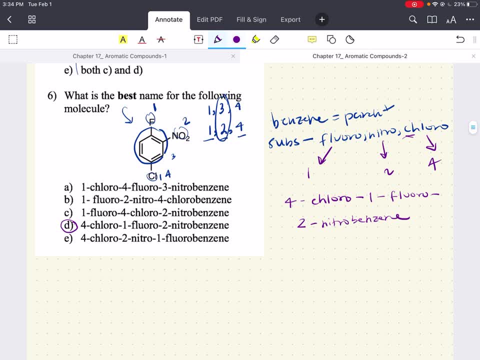 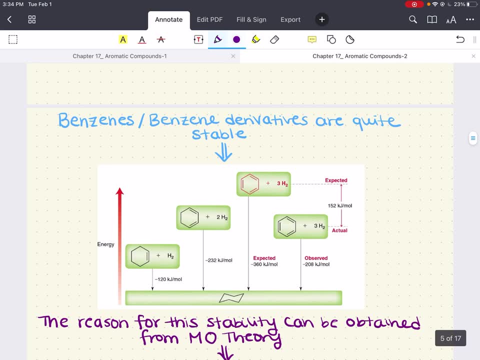 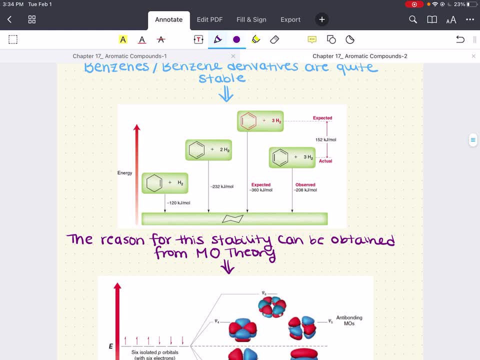 is also observed when comparing heats of hydrogenation for several similar compounds. Now, in order to explain the stability of benzene, we're going to need to invoke molecular orbital theory. So let's explore how molecular orbital theory describes the nature of benzene. 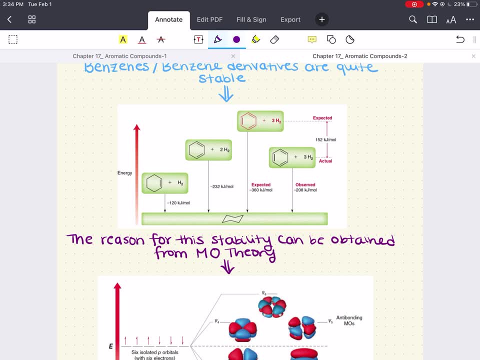 which is comprised of six overlapping p-orbitals. According to molecular orbital theory, these six atomic p-orbitals are replaced by the atomic p-orbitals. So if we look at the six molecular orbitals, we discussed this actually in detail last chapter, right? So? 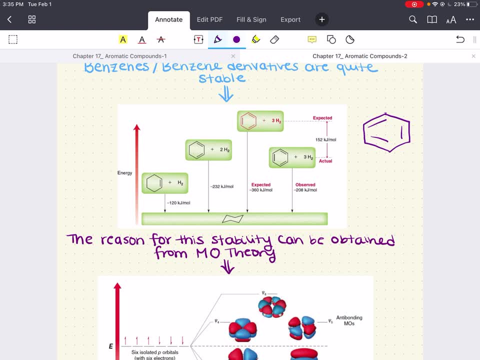 we have our benzene ring right here. All right, it's conjugated, All right, and there's a p-orbital here and here and here And, as you can see, there are six p-orbitals, six atomic p-orbitals, That. 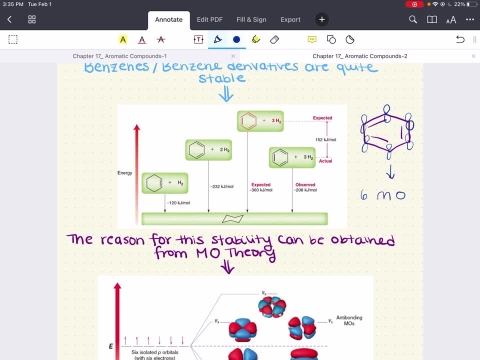 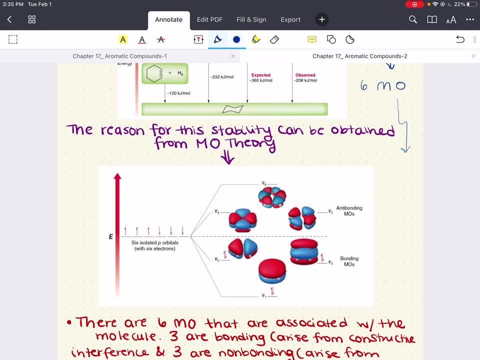 means this molecule has six molecular orbitals And you actually know how to draw this because we did an example, We've done examples of how to draw this, So we're going to draw this, So we're going to draw some examples on how to do this. All right, now, if we were to draw all six. 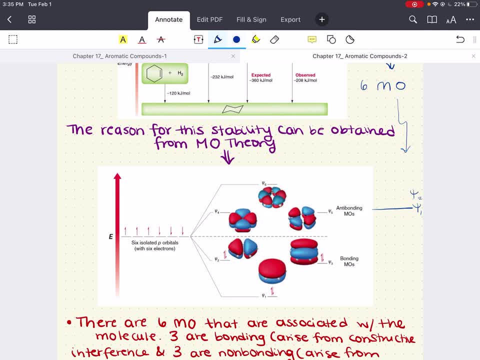 molecular orbitals for benzene, three, four, five and six. All right, we know how to do this. We could draw all six p-orbitals, All right. and then we know that at molecular orbital one here the lowest energy is going to have zero nodes. Two is going to have one, Three is going to have 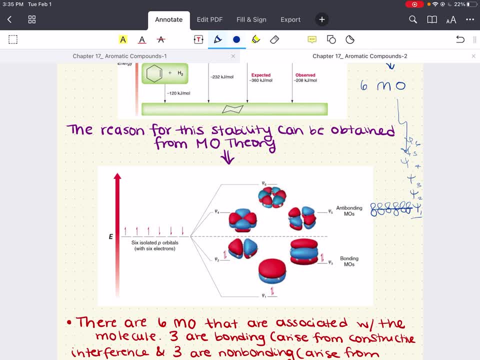 two, and so on and so forth. All right, and you can draw these out. What you realize is that three of the six molecular orbitals are going to be our bonding molecular orbitals. That means that they're going to be formed from constructive interference, while the other three 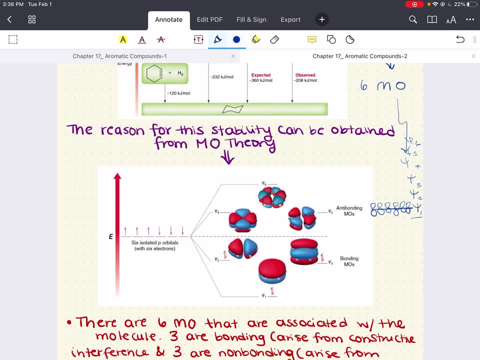 molecular orbitals are anti-bonding molecular orbitals. Now we have these six electrons from, obviously, our six p-orbitals. Since each molecular orbital can contain two electrons, right, the three bonding molecular orbitals can collectively accommodate all six of these electrons, Just following our. 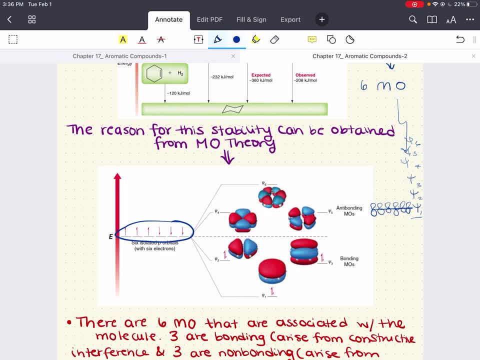 our Hund's rule, our Aufbau's principle and Pauli exclusion. all right, and we try to put in our six electrons, we notice that they're going to fill up all the molecular orbitals. All right, by occupying the bonding molecular orbitals, all six electrons are going to achieve a lower energy state. 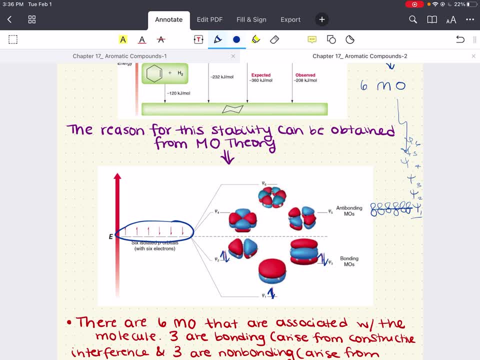 than occupying any of the anti-bonding molecular orbitals, and they're going to be delocalized Now, since the bonding molecular orbitals are filled with paired electrons, while the anti-bonding molecular orbitals are empty. benzene is said to have a closed shell configuration, and this 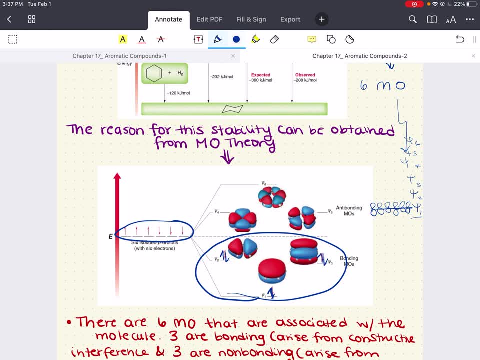 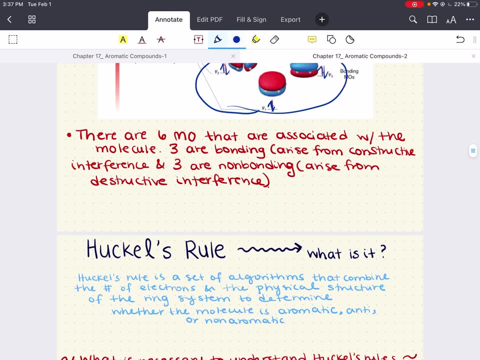 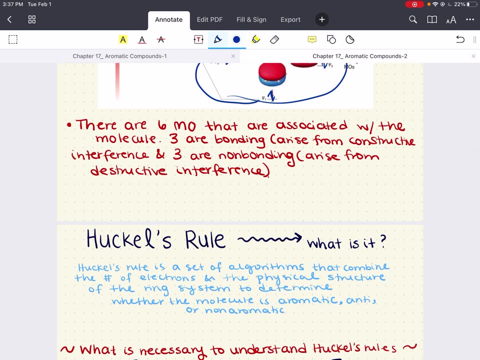 guys, is the source of the stability energy associated with benzene. Now we want to expand our understanding of aromaticity. This will also expand our understanding of the essence of of benzene stability. right Here we're going to learn about Huckel's rule. 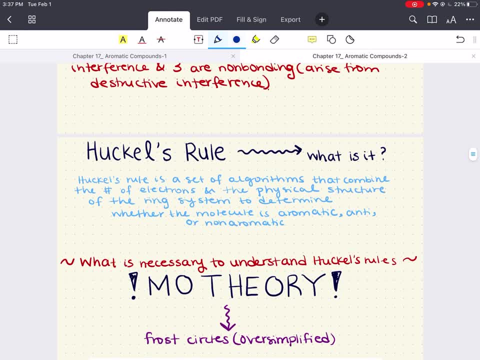 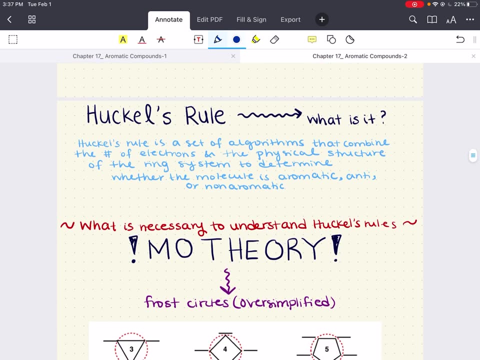 Huckel's rule is a set of algorithms that combine the number of electrons and the physical structure of the ring system to determine whether the molecule is aromatic, anti-aromatic or non-aromatic. Huckel's rule states that a compound can only be aromatic if the number of electrons, pi electrons- 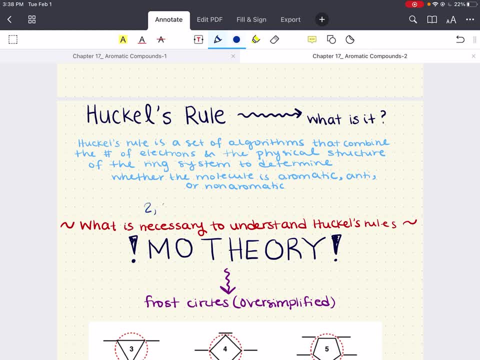 in the ring is either 2 or 6 or 10, anything that follows that you can get from the mathematical expression 4n plus 2, where n is a whole number, so it can only be 1,, 0,, 1,, 2,, 3, and so on. all right, 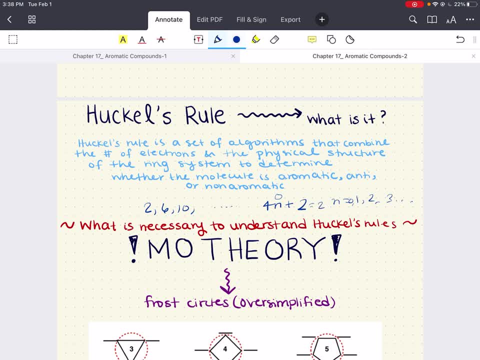 If you put in 0 for n, all right, you get 2.. If you put 1 for n, you get 6.. If you put 2 for n, you get 10, and that's how you figure out whether the number of pi electrons you have in a molecule is a Huckel's number or not. 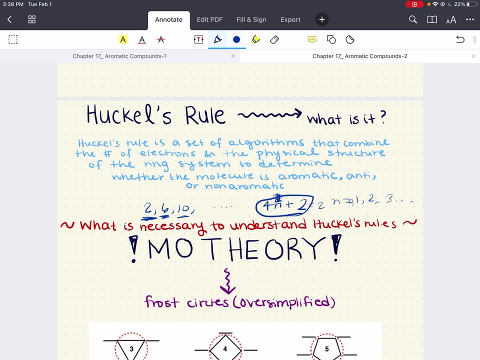 Can you get it from the 4n plus 2 mathematical expression. Now we will use molecular orbital theory to explain why aromatic stability requires this kind of number. Molecular orbital theory will also explain the source of Huckel's rule for planar conjugated ring systems, and this will 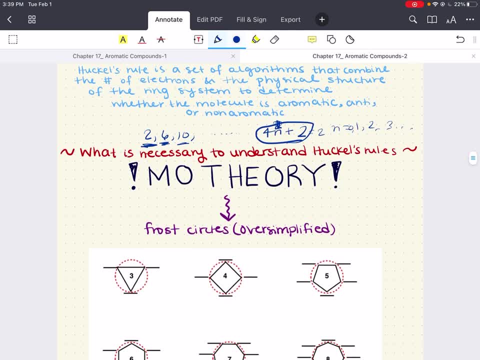 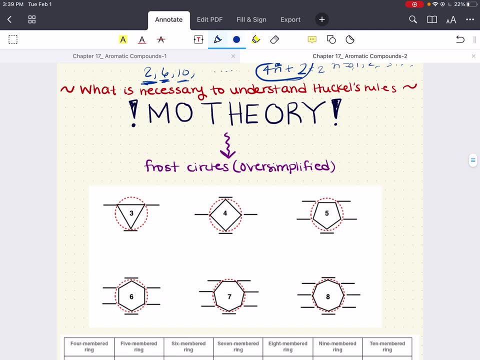 make more sense in just one second. Now. the way we will convey this point ultimately is using frost circles. Whether or not a compound is aromatic may be determined by the so-called frost circle. It's a simple method. It's used to estimate the relative pi orbital. 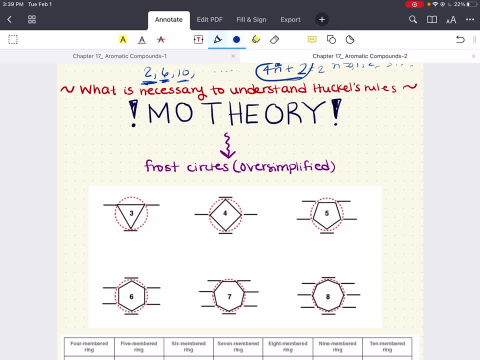 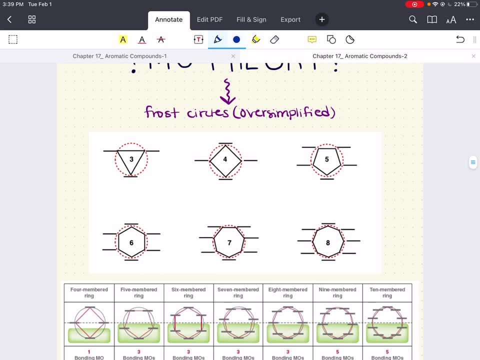 energies of both planar cyclic compounds with uninterrupted pi electron systems. So, to begin with, the structure of the cyclic compound you're working with is placed inside a circle with one of its vertices pointed. So if you're working with a cyclic compound, you're going to have to. 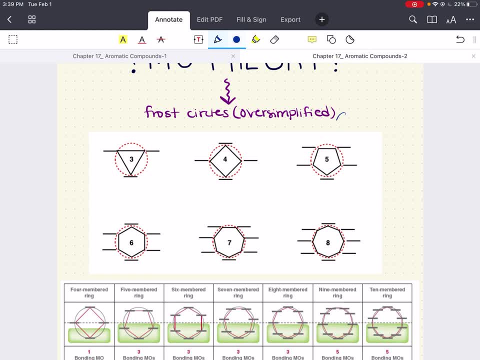 draw a 5-membered ring. This is our 5-membered ring. We draw it with one of the vertices pointing downward. It's encompassed within a circle. A short horizontal line is then added to each of the molecular structure's vertices, along with a horizontal dashed line. that's going to run right. 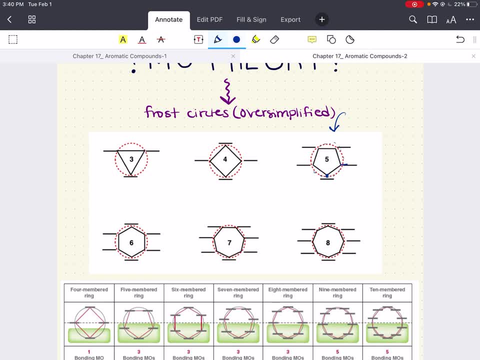 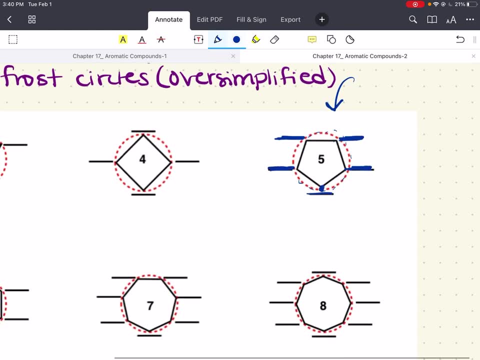 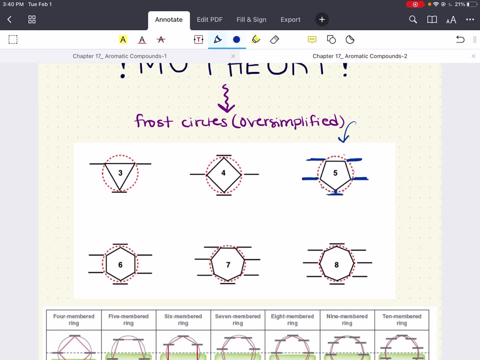 through the center. For every corner of this 5-membered ring we're going to draw a straight horizontal line, as you see here. The reason we do this is because this conveys the number of molecular orbitals for this ring. So for a 5-membered ring we expect: 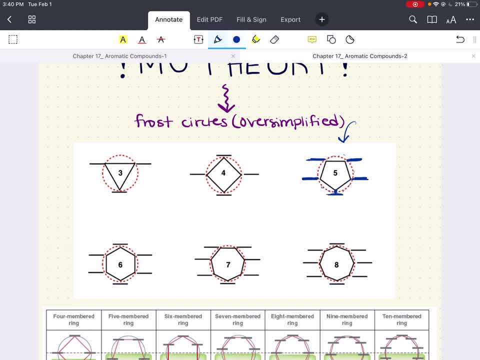 5 molecular orbitals. Alright, then, what we want to do is we're going to draw a line right through the center of this horizontal line. What we can determine from this, then, is the number of physicians that really have this hard core, because our 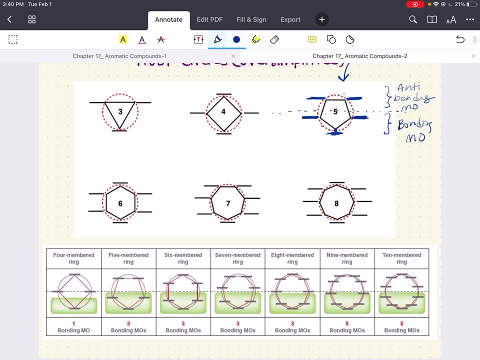 sequence of molecular fights the entire Hungarian collection and often throw the theresflix park store. So we now plot at least 40 of those two views. The strikeup is from the 1-membered ring. If we dig through to the left again, kinds ofgenes apart, let's refer to our molecular orbitals. 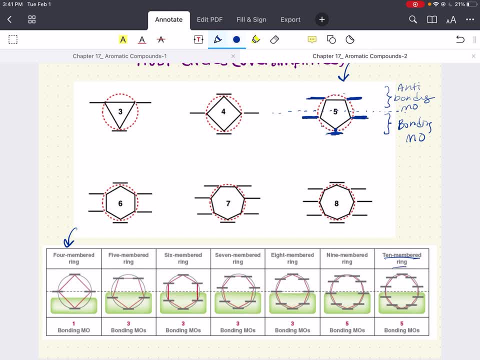 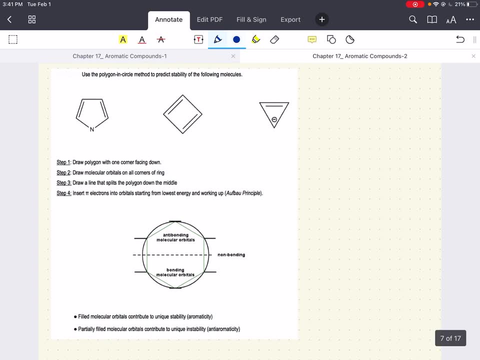 this very well, from four-membered rings all the way to ten-membered rings. all right, Now here is also a step-by-step guide that's really going to help us here, all right. So how do you do frost circles for different size-membered rings? all right, You're going to draw the polygon. 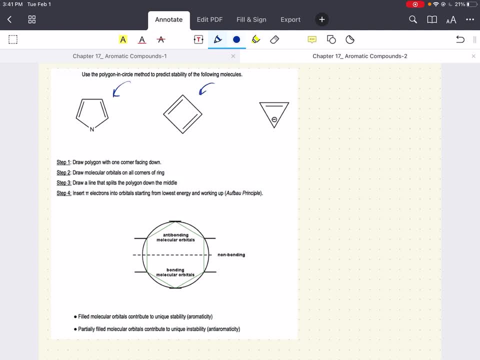 whatever, it is all right, with one corner facing down. So if you have a four-membered ring, at least have one vertice pointing downward and you're going to encompass this within a circle, all right. Then you're going to draw molecular orbitals on all the corners of the ring. Here's 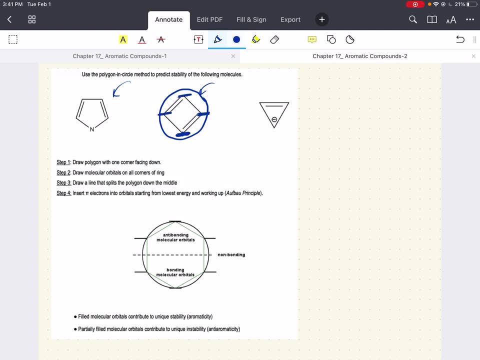 all our corners, Fantastic. And then you're going to draw a line that splits the polygon down the middle. Anything below the line is our bonding MOs. Anything above the line is our anti-bonding MO. If you happen to come across like, for example, this is a great example where 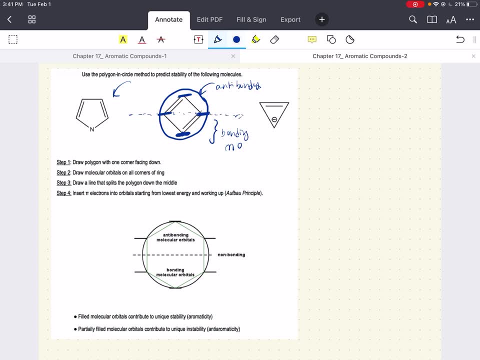 you have molecular orbitals on the dashed line. These are actually just your non-bonding MOs, all right, And then you're just going to whatever, however many pi electrons you have, you're going to go ahead and fill them in from lowest energy working up. 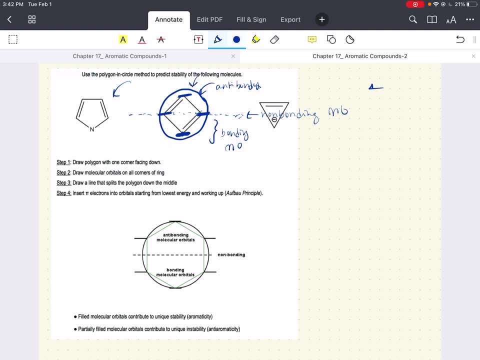 all right. So this four-membered ring with two double bonds has four total electrons. all right If we fill them up. one, two, all right, three, four. we realize that we are filling up some of these non-bonding MOs. 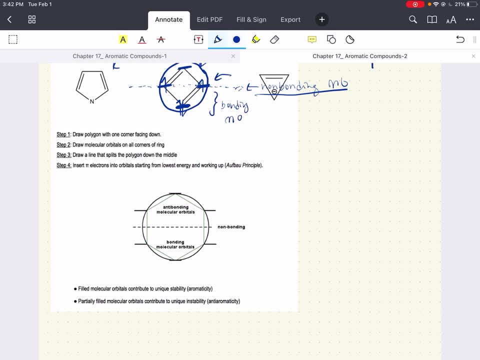 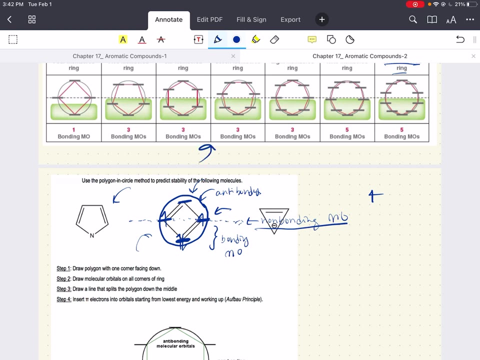 All right, This is going to make a lot more sense when we elaborate on how to determine whether something's aromatic, non-aromatic or anti-aromatic. So keep this example in mind. But generally, whenever you're practicing this, this diagram is a great thing to reference back. 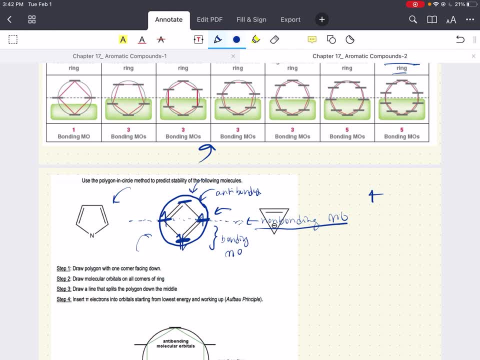 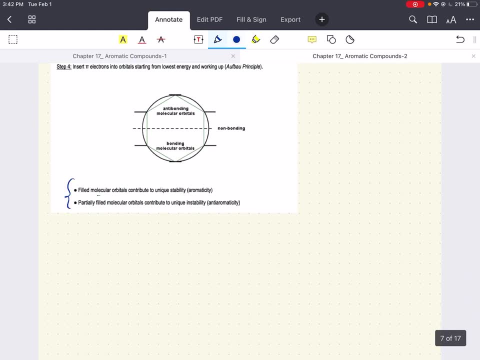 to make sure you understand how to draw frost circles for any numbered membered ring. All right, fantastic. Now two notes to keep in mind. Filled molecular orbitals contribute to unique stability- all right. or aromaticity: Partially filled molecular. 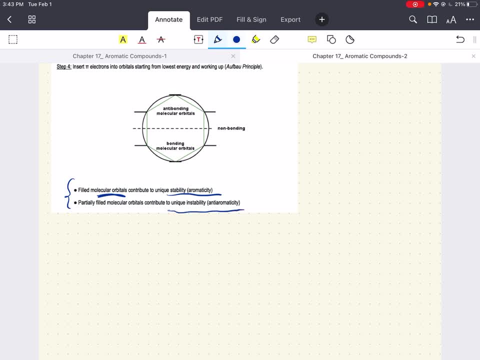 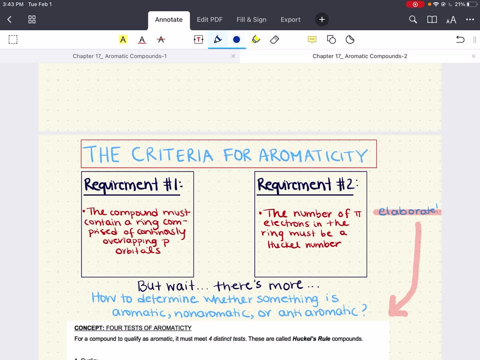 orbitals contribute to unique instability or anti-aromaticity. Fantastic. So so far what we have said. we have said that the criteria for aromaticity is that a compound must contain a ring comprised of continuously overlapping p-orbitals and that the number 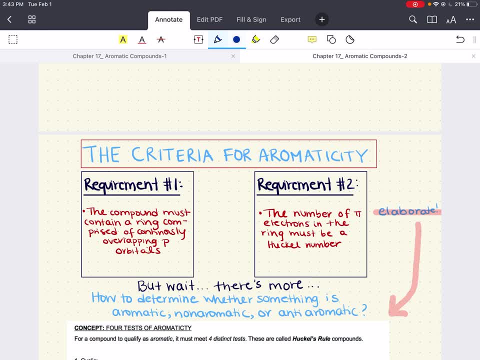 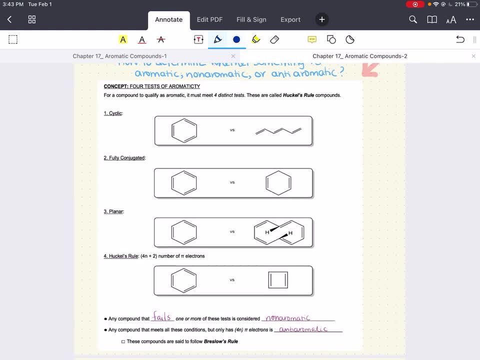 of pi electrons in the ring must be Huckel's number. Let's turn this into an actual step-by-step guide and elaborate. So this is a really awesome diagram I found on Clutch Prep. They have, like these blank notes that you can download for free. 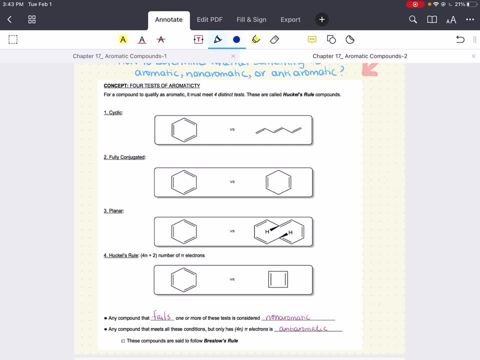 and I found this on their website. It states that for a compound to qualify as aromatic, it must pass these four criteria. All right, they're called Huckel's rule. All right compound, All right. so the first first thing that your molecule has to meet is that it must be cyclic for it to be aromatic. 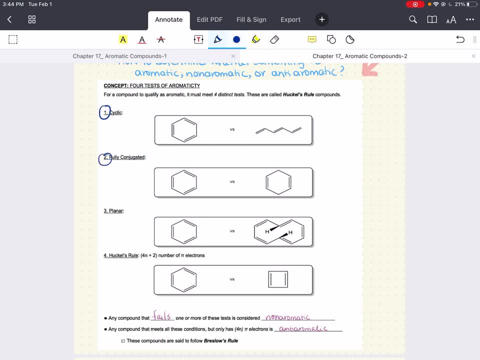 It must be fully conjugated, it must be planar and then it must have a Huckel's number of pi electrons. All right, so if your molecule meets all four criteria, then it is aromatic. Now, if any compound fails one or more of these tests, 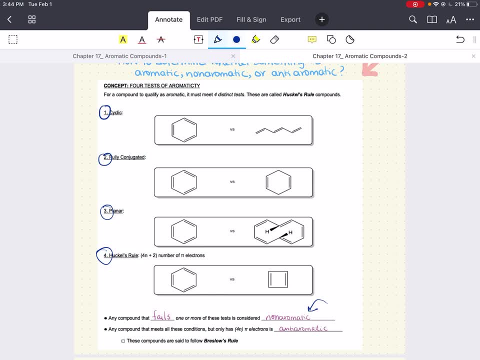 all right, it's considered aromatic, Non-aromatic. Any compound that meets all these conditions- one, two and three- but it has four n pi electrons as opposed to four n plus two, as Huckel's rule states, then it is anti-aromatic. 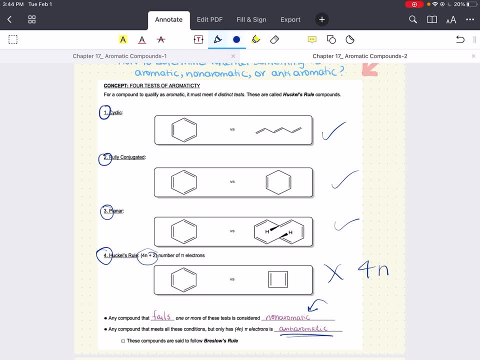 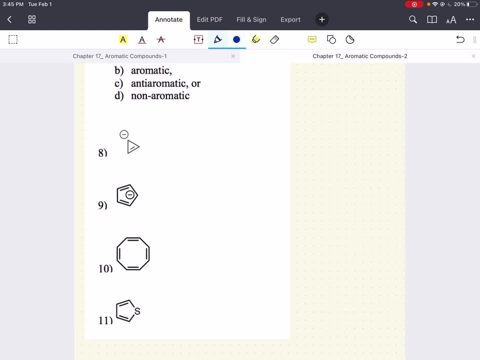 All right, so that's a good thing to keep in mind. Now, with that being said, let's do some practice problems so we can really understand this. All right, looking at our first question, example here is this: aromatic, anti-aromatic or non-aromatic. So let's go through our steps. 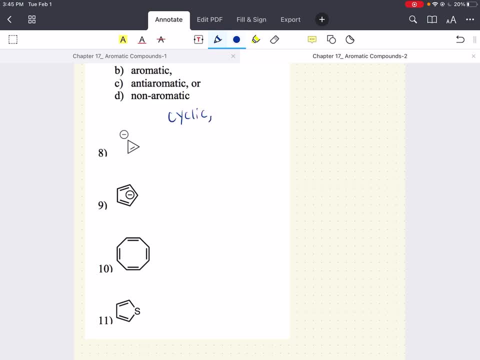 This is obviously a cyclic molecule. It's conjugated right. This negative charge refers to a lone pair that sits in a pi orbital, and then these double bonds also have pi orbitals, so there's three overlapping p orbitals. This molecule is conjugated Fantastic. 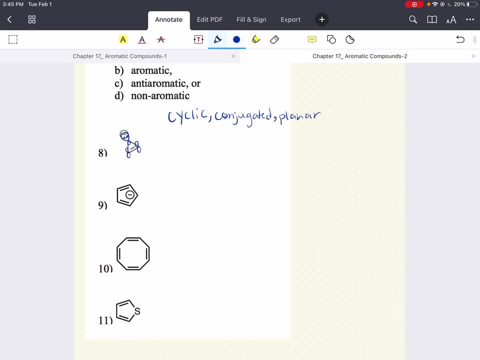 It's also planar. There's no wedges or dashes sticking out of the page to indicate otherwise. All right, but now how many pi electrons does it have? It has two from the lone pair, all right, and then two from the double bond. This molecule has four pi electrons. Four. 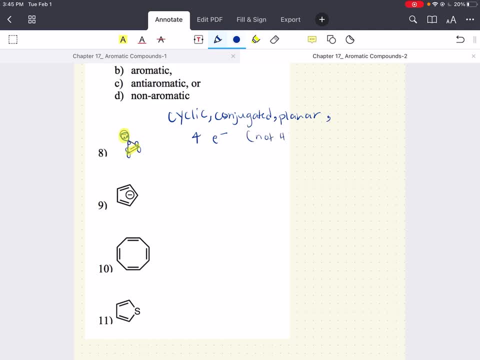 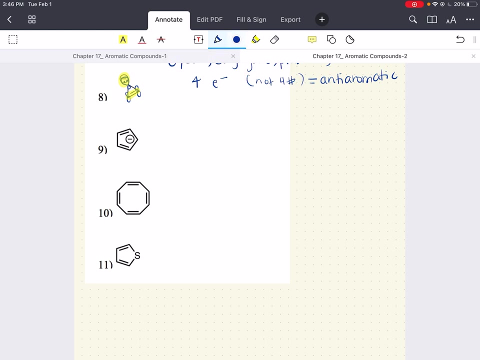 is not a Huckel number. All right. so it meets the first three criteria, but it doesn't have a Huckel number. This molecule is anti-aromatic. All right, let's do nine. All right, let's look at this molecule. It's cyclic. Is it conjugated? There's a p orbital here. 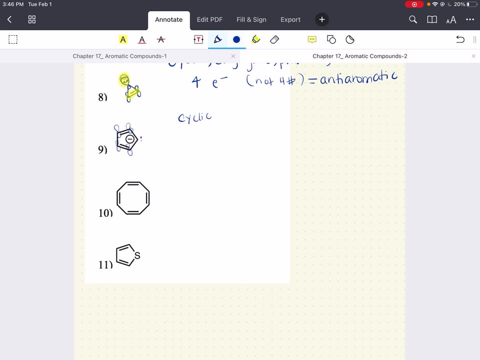 here, here and here, and then this negative charge indicates there's a lone pair here that's sitting in a p orbital. All right, it's also conjugated. All right, it's planar. We don't see any wedges or dashes indicating otherwise. Fantastic. Now let's count how many electrons. 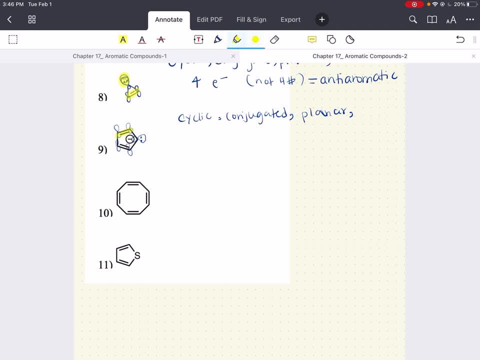 this how many pi electrons this molecule has? Two from this double bond, two from this double bond and two from the lone pair. That's a total of six pi electrons. This is a Huckel number. All right, this molecule meets all five criteria. 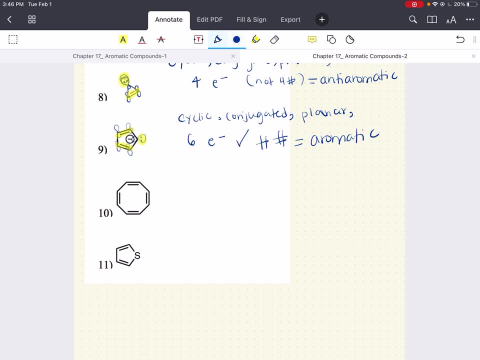 to be an aromatic compound. Fantastic. Let's do this next one here. All right, it's cyclic, It's conjugated. There's eight overlapping p orbitals here. All right, draw them out for each of the double bonds. All right, it's also planar. No wedges or dashes indicating otherwise. Let's. 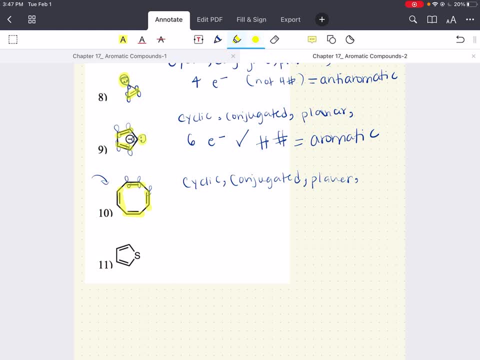 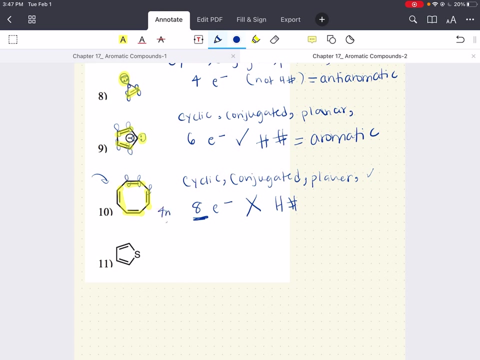 count the number of electrons: Two, four, six, eight. This molecule has eight pi electrons. This is not a Huckel's number, All right, so it meets the first three criteria, but it has four n electrons. right Four n If n was. 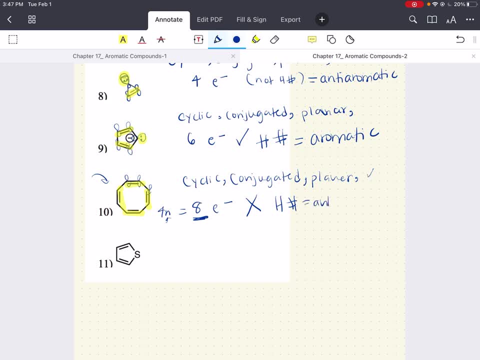 two, that would equal eight. So this is anti-aromatic, just like the first one we did. All right. now let's do this last one. All right, this is cyclic. It's also conjugated. This is sulfur. All right, on the periodic table we have four n electrons, So this is anti-aromatic. This is. 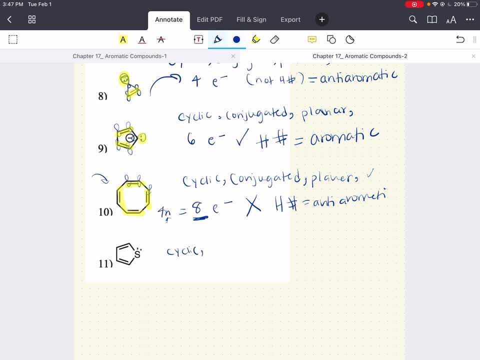 a periodic table that's right underneath oxygen. It has a similar idea in terms of it likes to form two bonds and have two lone pairs. One of these lone pairs sits in a p orbital right, And that means this molecule is indeed conjugated. All right. it's also planar, And let's count how. 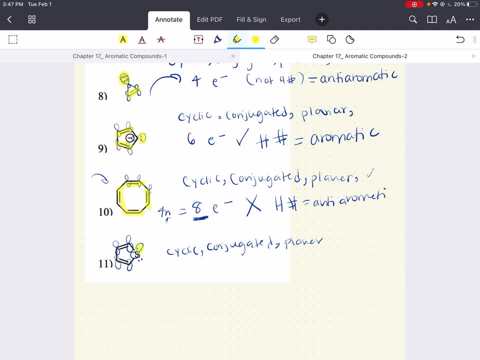 many electrons. there are here Two from the sulfur, the lone pairs there, Two for this double bond and two for this. That's six total electrons. That's Huckel's number Fantastic. So this makes this molecule- it meets all four criteria. It is 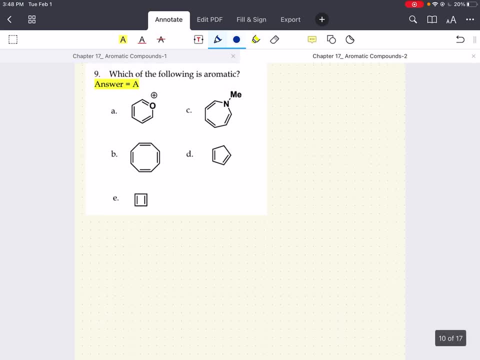 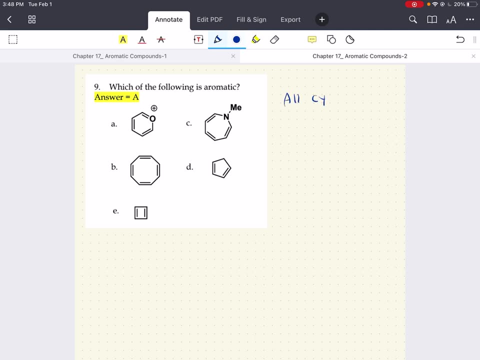 aromatic, Fantastic. Let's do one more practice problem on this. Which of the following compounds is aromatic? Now, they're all cyclic, All right. so let's move on to our next criteria. Are they all conjugated? All right? A has p orbitals all around here. the double bond. Here oxygen has a. 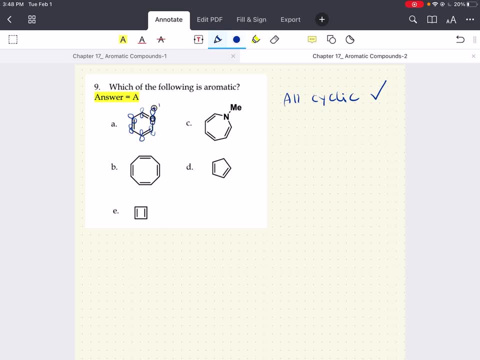 positive charge. It has this empty p orbital here. All right, this molecule is conjugated. This molecule is also conjugated. You have all these p orbitals, All right. and the lone pair on nitrogen here sits in a p orbital as well. Remember a no charge. nitrogen forms three bonds. 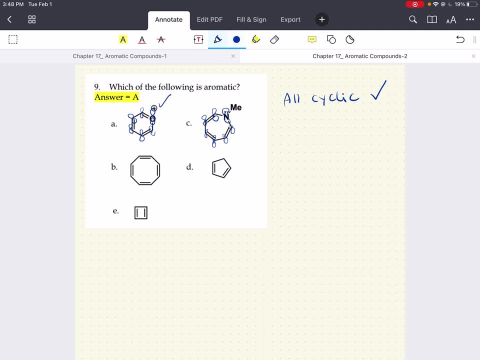 and it has one lone pair. That lone pair is sitting in a p orbital. This is also conjugated. We just did this, something similar to this. right, There's p orbitals all around. This is also conjugated. Now, if we look at D, 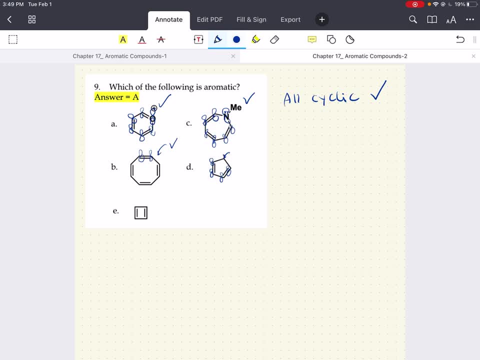 D is not conjugated. We're missing a p orbital here. that isn't there, So this is not conjugated. All right, this. however, E is also conjugated, So four out of these five answer choices are conjugated. We can throw D out completely. All right, so we've gone through cyclic, We've 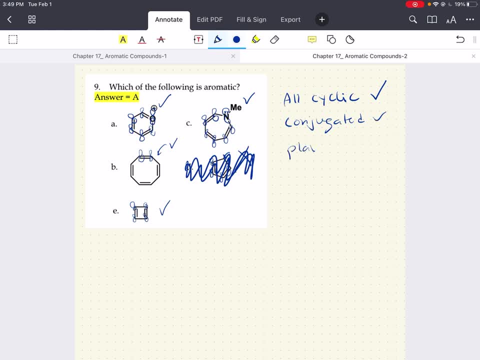 gone through conjugated, They're all planar. The four that we have left, they're all planar, no wedges or dashes that indicate Otherwise. now we have to count our electrons. All right, we're going to count our electrons. So if we look at A, let's erase these. 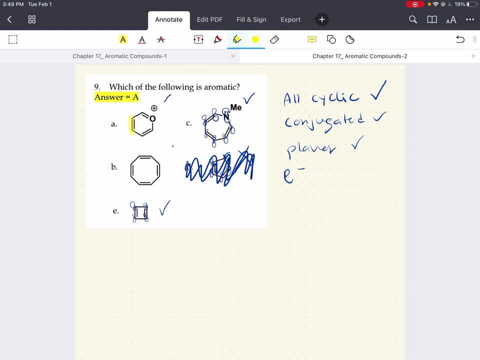 p orbitals. so we can count properly. A has two, four, six electrons. C has two, four, six, eight electrons, Those two lone pairs on the nitrogen we have to count, All right. B has two, four, six, eight electrons here, All right. and then E has two, four electrons. 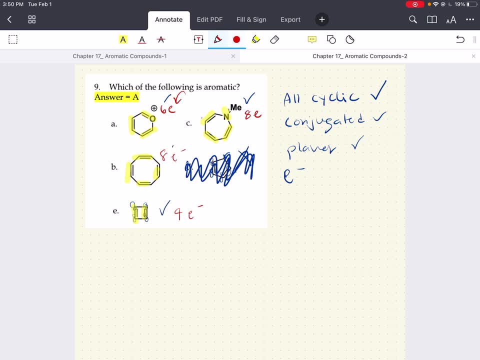 Answer choice that has a Huckel number of pi electrons is A. So the only molecule that is aromatic here is answer choice A. All right, so always make sure to ask yourself: is it cyclic, Is it fully conjugated, Is it planar, And does it follow Huckel's rule for number of electrons? 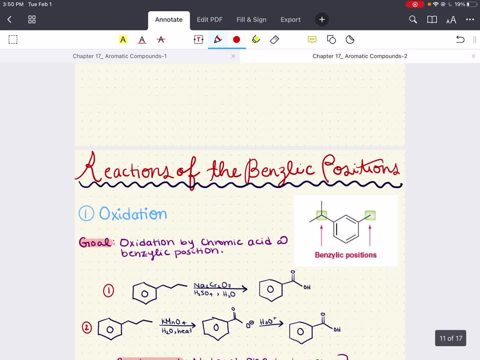 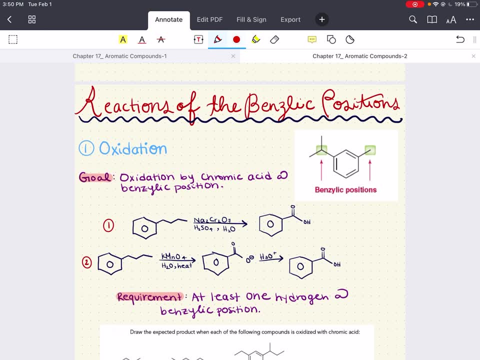 All right now. with that being said, we're going to move on to reactions at the benzylic position. First, let's note what constitutes a benzylic position by looking at this image right here. Here's our benzene ring. All right whenever we have a substituent coming out. 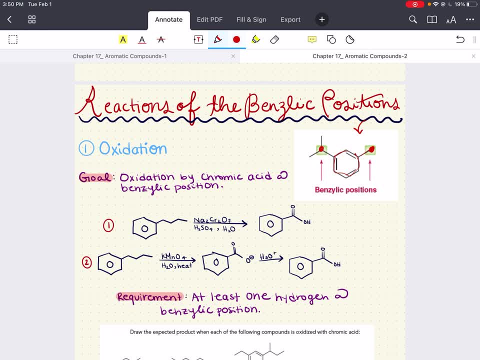 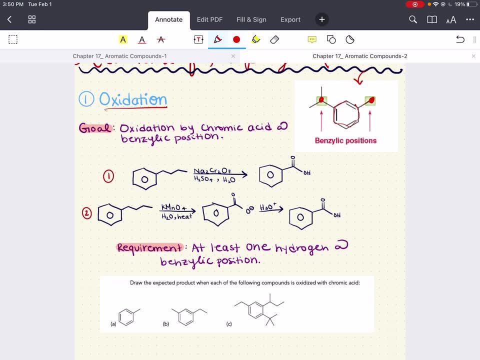 all right. this next atom off of our substituents are our benzylic positions. Now, the first reaction we're going to be talking about is oxidation. Alkyl benzenes are readily oxidized by chromic acid. The oxidation is going to take place selectively. 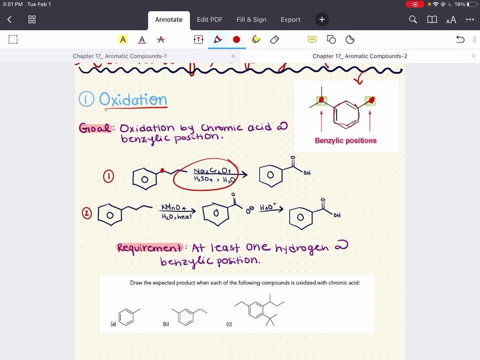 At the benzylic position. the only condition it requires is that there's actually hydrogen at this benzylic position. All right, so if you have a hydrogen at your benzylic position, you can then treat it with chromic acid, And what happens is this gets oxidized and you form 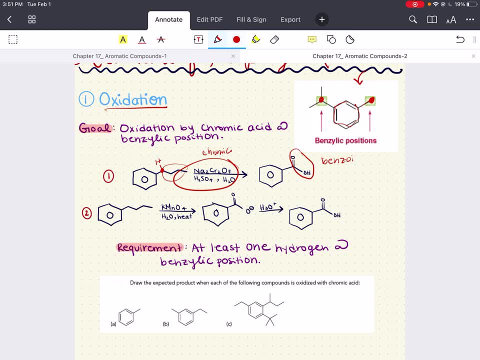 a benzoic acid. You have a carboxylic acid right here and this becomes benzoic acid. All right, you can also do this. There's another way to oxidize benzylic position: You can treat it with potassium permanganate and then you're. 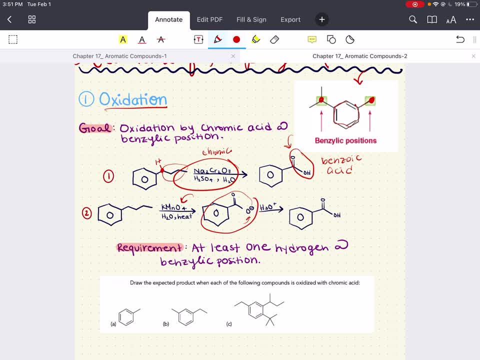 going to form this carboxylate salt, right, because you have this negative charge here, And then you can protonate that obviously with, say, H3O, All right, and then you get again your benzoic acid, All right. so that's another way to oxidize your alkyl benzyne. 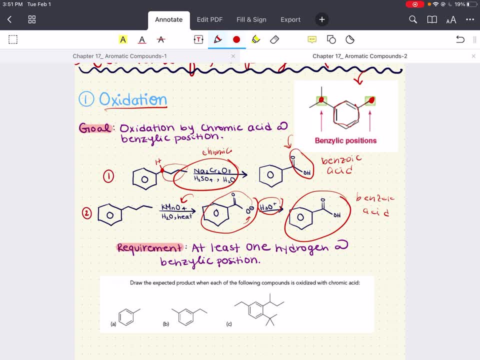 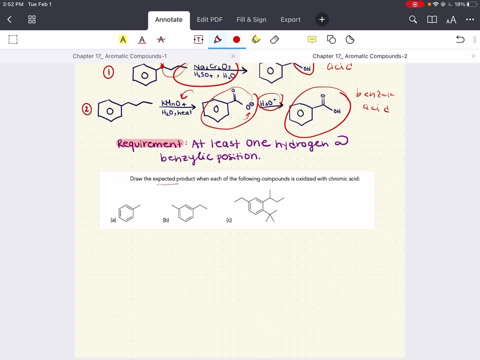 All right. potassium permanganate with some source for your proton like water or hydronium, All right. so let's go ahead and just do some examples. Draw the expected product when each of the following compounds is treated is oxidized with chromic. 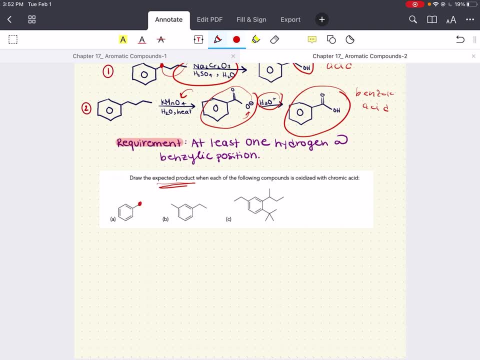 acid. So we'll look at A. We have a benzylic position right here and guess what? It has at least one hydrogen, So it will successfully oxidize to give us a product that looks like this benzoic acid. Fantastic, All right. 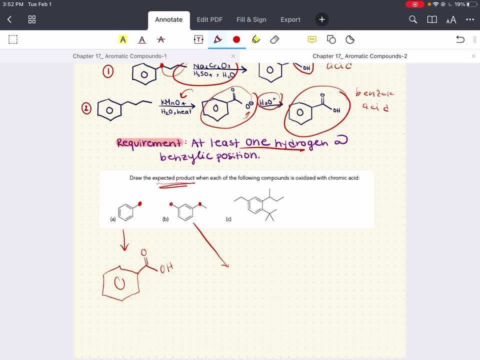 let's look at B. B has two benzylic positions and guess what? Both of them have hydrogens, at least one hydrogen. All right, if we're going to treat it with chromic acid, both of those benzylic positions are going to get oxidized, not just one. 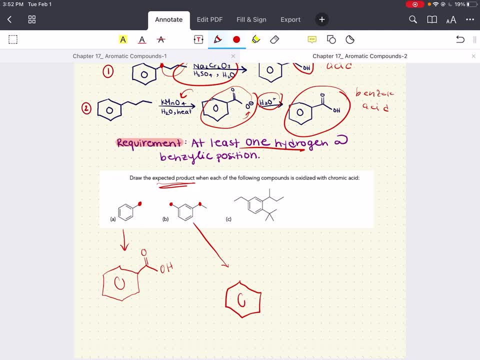 So our product is going to look like this: Fantastic. Now let's look at C. C has three benzylic positions. Only two of them, though, have hydrogens there. So what that means is we're only going to oxidize these two positions. This one stays as is because there are no hydrogens. 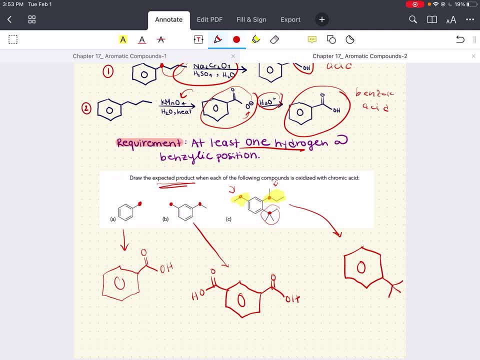 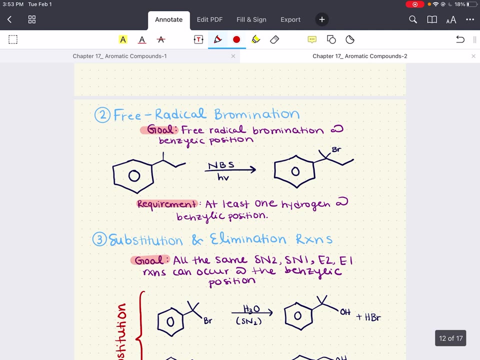 So we're going to go ahead and draw it. We keep the tert-butyl group. It doesn't get oxidized. This gets oxidized, however, and so does this position. So, therefore, this is our final product- Fantastic. Now, what we want to talk about is the second reaction. The second 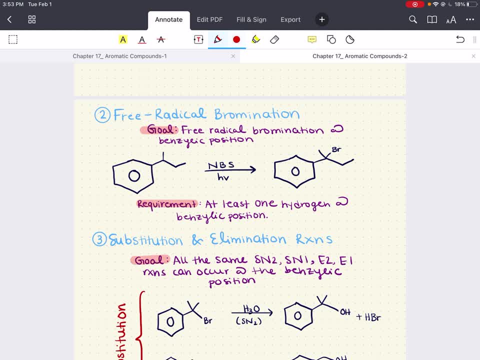 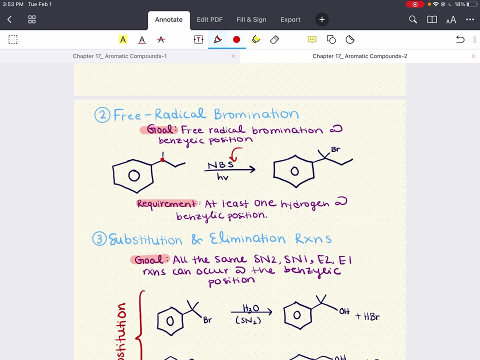 reaction we're going to discuss is free radical bromination, All right. if there is at least one hydrogen at the benzylic position, then we can add bromine there using NBS, All right. so if we have a benzylic position and the requirement here is there's at least one hydrogen, all right. 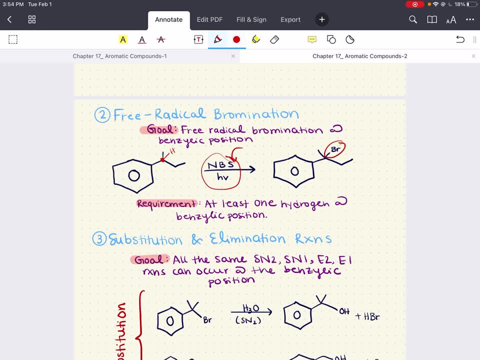 we can treat it with this To add a bromine here. Now, this is going to be a really important kind of reaction that we'll use when we're doing synthesis-based problems. that we'll get to in a second. All right, now the 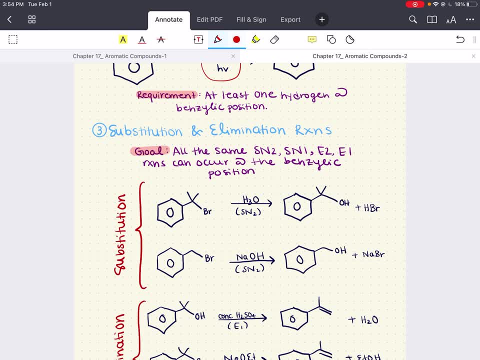 third reaction, or let's say set of reactions we want to discuss that we can do at the benzylic position is our normal substitution and elimination reactions. All the same, SN1,, SN2,, E2, and E1- reactions we covered in chapter seven of organic chemistry. 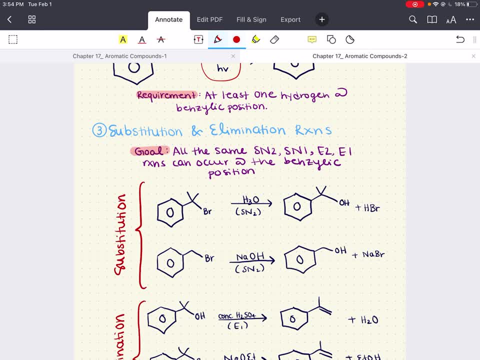 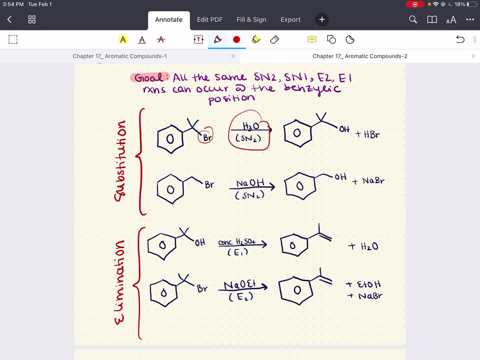 here, All right, and here are a few prominent examples: All right, whenever you have a bromine here at the benzylic position, you can treat it via SN2 with hydronium and convert the bromine to an alcohol group. All right, or sodium hydroxide as well, and convert that bromine to an alcohol. 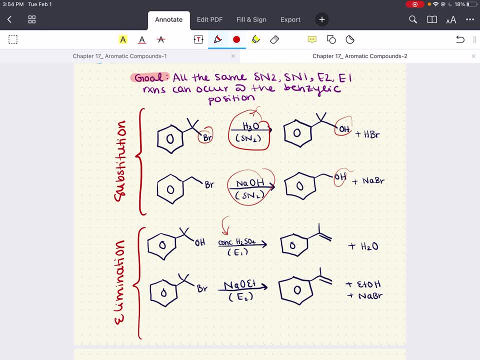 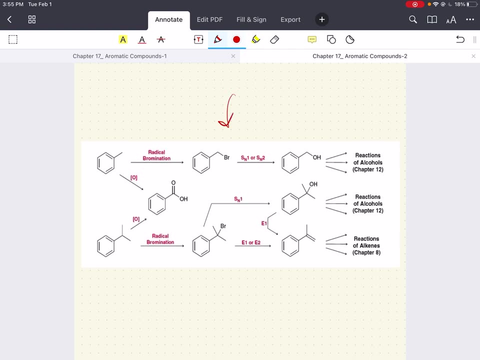 group. You can also treat a benzylic position with concentrated sulfuric acid or sodium ethoxide to form double bonds. These are going to be really important again, like I said, for synthesis problems. All right, here's a nice diagram from David Klein that kind of summarizes all these reactions we've talked. 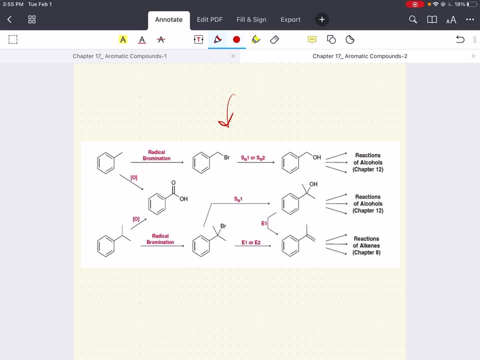 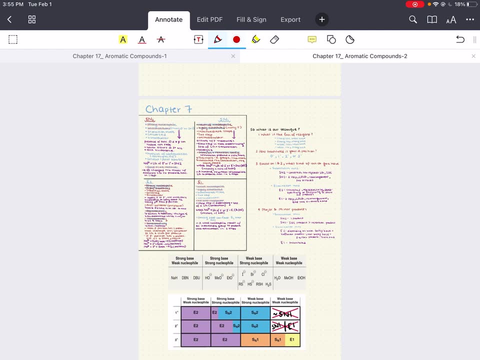 about and how to interconvert between molecules and compounds. All right, and also here I've embedded a page summary of my chapter seven notes. All right, if you've forgotten how to do substitution and elimination reactions, you can go ahead and watch my videos for that. just to: 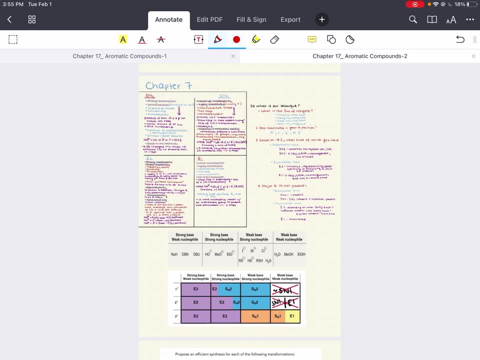 refresh. They will be important for the rest of organic chemistry too, Because you'll continuously be doing synthesis problems within every chapter starting from now. All right, so it's good to re-familiarize yourself with here. I have quick notes on every reaction. 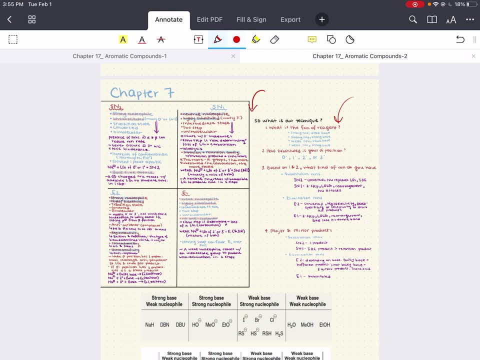 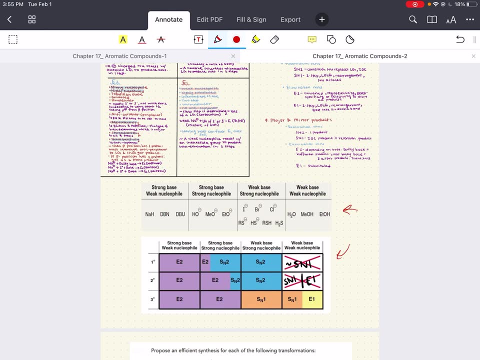 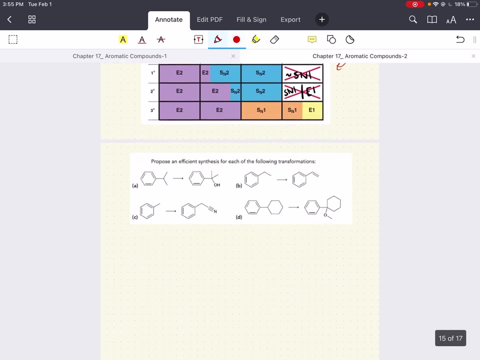 over here. All right. your technique, excuse me. All right, and these two tables that are very important, All right. so if you need to refresh, go ahead watch my videos, and here's a key page that summarizes pretty much the whole chapter as well. All right. so, with that being said, 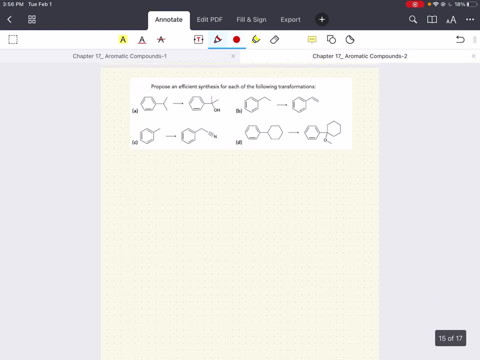 let's actually do some practice synthesis questions, All right. so starting here with A: All right, this is our starting molecule. All right, and we want to convert it to something that looks like this: that has this alcohol group added. All right, now we know how to add groups, We know how to. 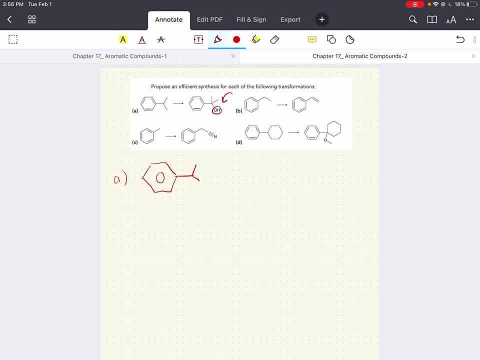 substitute groups, especially good leaving groups, all right into other groups that we want. So, for example, if we had a good leaving group here, say, we can easily do this, We can do this with an alcohol group, but the problem is we don't have any leaving groups right now. So the first step we 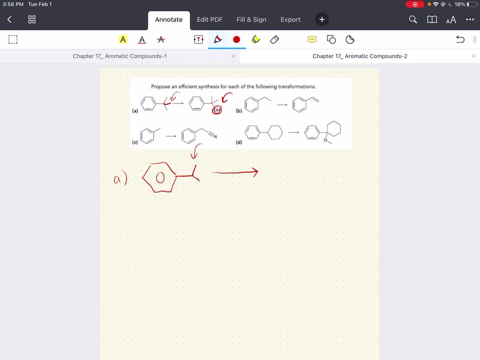 should do here is add some sort of leaving group, and we know how to do this, because we just talked about free radical bromination, So using NBS- excuse me, we can add a bromine there. All right, now that we have our bromine, we can do a normal substitution. 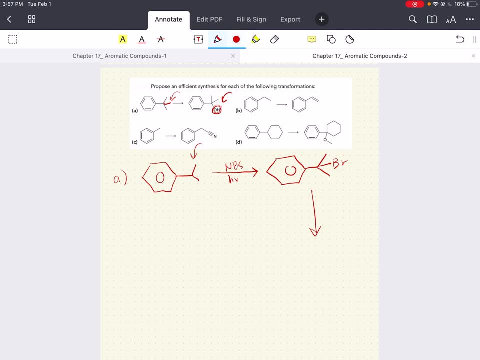 Reaction and change that bromine into an alcohol group using just water, All right through SN1.. Excuse me, I'm still recovering from COVID, so I still have a bit of a cough. All right, so there we go. Now we have our alcohol group. Fantastic, Let's do another problem. 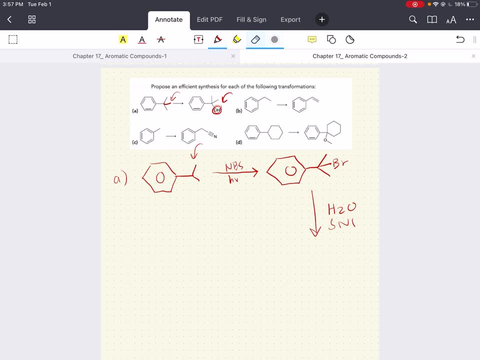 Let's do B. All right, let me just make some room here. Here's B. All right, look at this. We want to go from this into something that has a double bond. right there, We know how to do this through an elimination reaction, but once again, 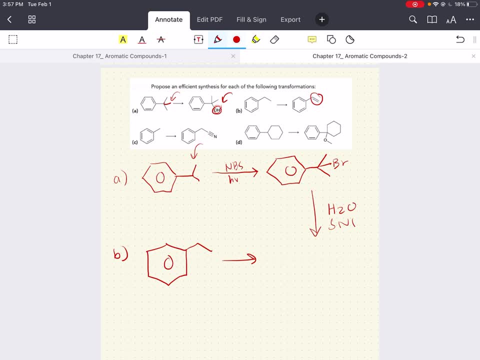 we need a leaving group in order to do this. So we're going to go ahead and once again use our NBS trick here to add bromine at the benzylic position And once we have our bromine there, once we have our bromine there, we can go ahead and just use a base like sodium ethoxide. 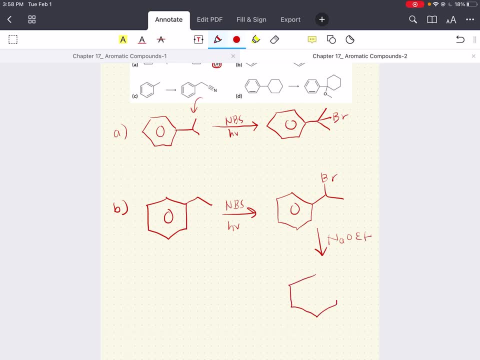 To go ahead and convert it to a double bond, right? Our ethoxide is going to come steal this hydrogen, It'll dump its electrons here and we'll form that double bond we want. All right, so this is how you want to approach these synthesis questions. Go ahead and make an attempt at doing. 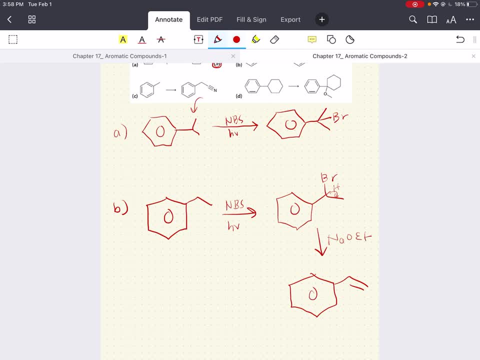 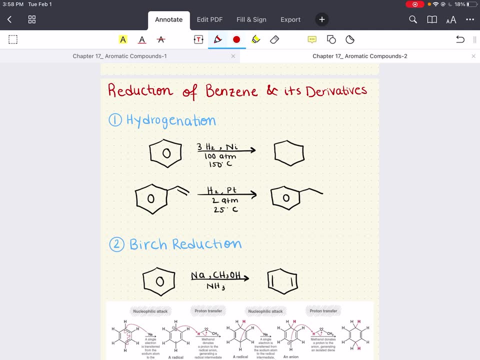 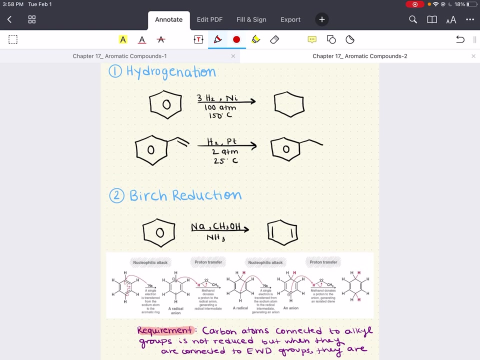 C and D yourself, and let me know if you have any questions or problems figuring it out. With that being said, we're going to move into our last topic. here We're going to want to cover reduction of benzene and its derivatives. All right, the two main reduction reactions we're going to elaborate on are hydrogenation. 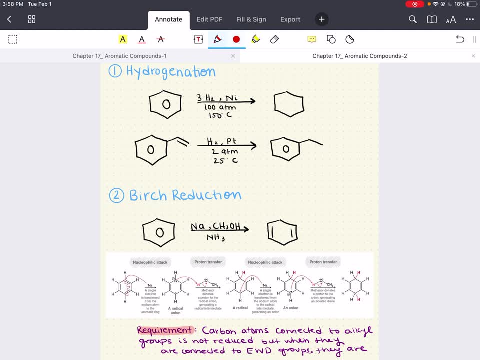 and Birch reduction. Now for hydrogenation. all right, under forcing conditions. benzene can react with, say, three equivalents of molecular hydrogen with some sort of catalyst like nickel to completely hydrogenate this ring and you'll form a cyclohexane. All right, now, with some catalysts. 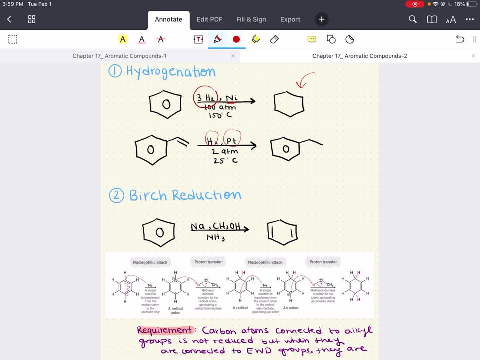 and only one equivalent of molecular hydrogen. we're going to want to elaborate on hydrogenation like this and say platinum. it's possible to selectively hydrogenate a venial group in the presence of an aromatic ring. So with just one equivalent of molecular hydrogen and a catalyst. 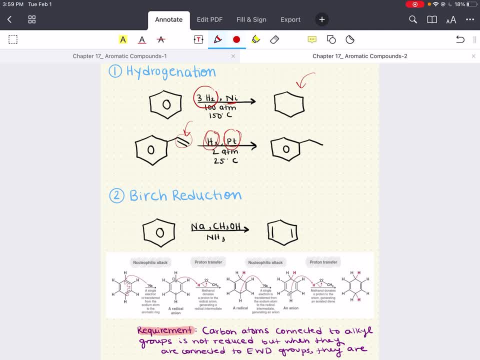 like platinum, we can simply hydrogenate just this double bond and keep our aromatic ring, And that is really important. These two are really important for, again, synthesis problems. All right, you might want to only hydrogenate like a venial group, for example. 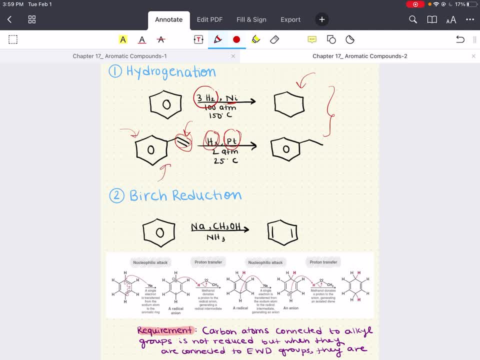 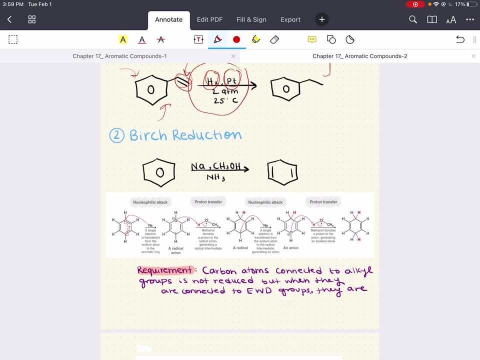 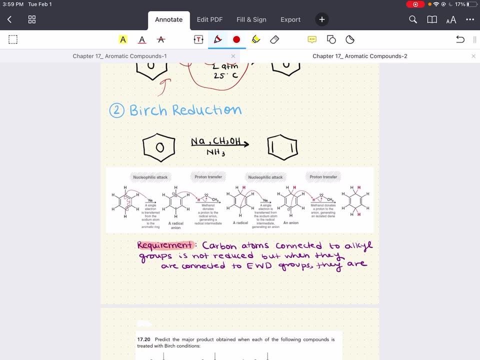 all right, and keep your aromatic ring Well. using less equivalents of molecular hydrogen and certain catalysts you can do that. So that's a good thing to keep in mind for future synthesis problems. Now for Birch reduction. recall. recall back in chapter eight of organic chemistry one. 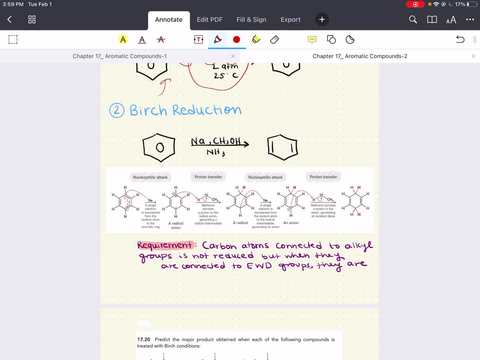 you know we talked about how alkynes can be reduced via the dissolving metal reduction. All right now benzene can also be reduced under similar conditions to give us 1,4-cyclohexadiene. This reaction is called Birch reduction, And here's the 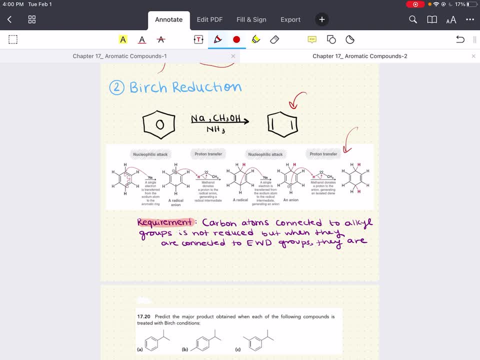 mechanism for Birch reduction. you'll recognize it's pretty similar to the dissolving metal reduction. Now the product of a Birch reduction is a non-conjugated diene rather than a conjugated diene, And whenever you have an alkyl benzene and you treat it with Birch condition. 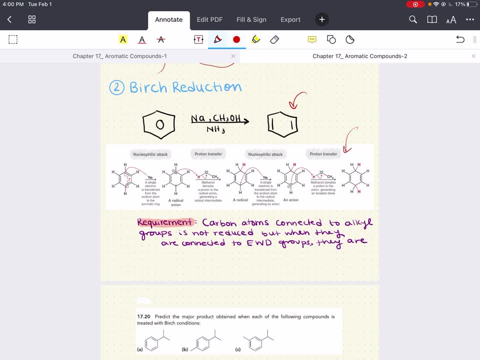 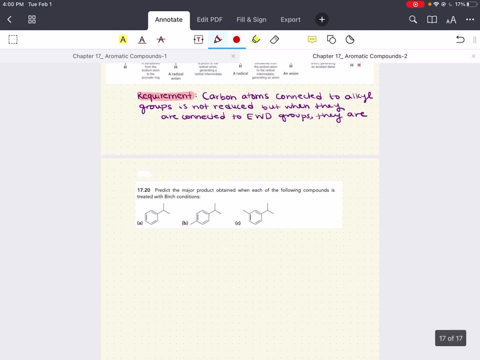 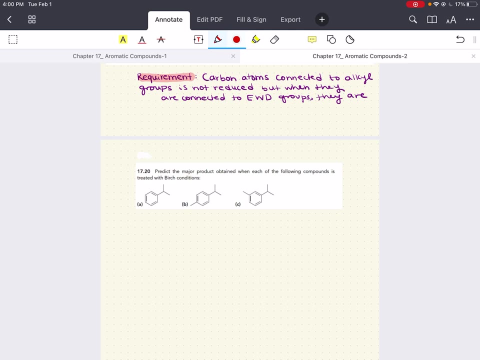 all right. the carbon atoms connected to alkyl groups are not reduced because they are electron donating, All right. so we're going to see this in some example problems: Whenever you have some alkyl benzene, you have some hydrocarbons substituent to your benzene, the carbon 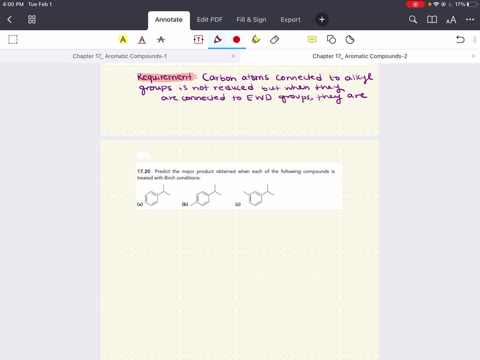 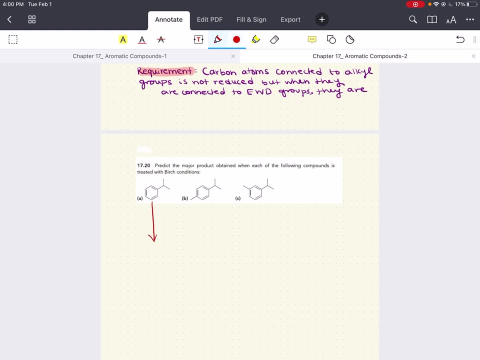 that is attached to that is not reduced. So you must keep that in mind. Whenever you take a material like this, treat it with Birch conditions and try to draw the final product. So if we look at the starting material, at this carbon, 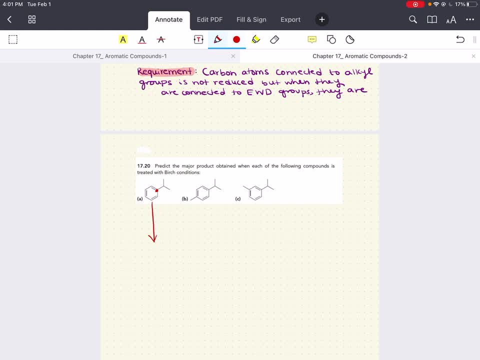 we have an alkyl group, All right. that means that this carbon is not reduced. That means that double bond has to stay. That double bond is still there, All right. and that makes it easy, though, for us to draw the final product after Birch conditions, because we have our 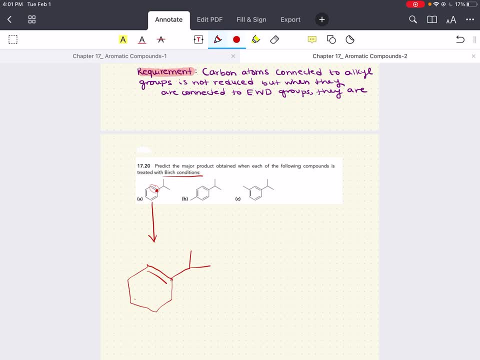 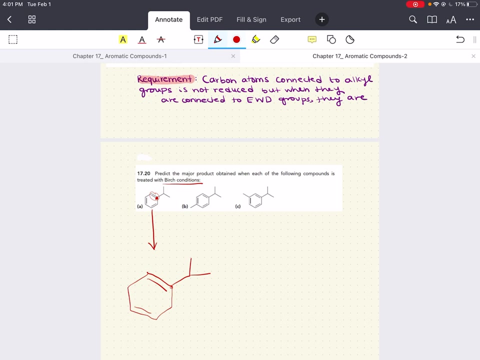 double bond here. this carbon isn't reduced, All right. and we want to treat it. we want to form it into this 1,4-hexadiene- Oh, my God, it slipped my mind. 1,4-cyclohexadiene, All right. 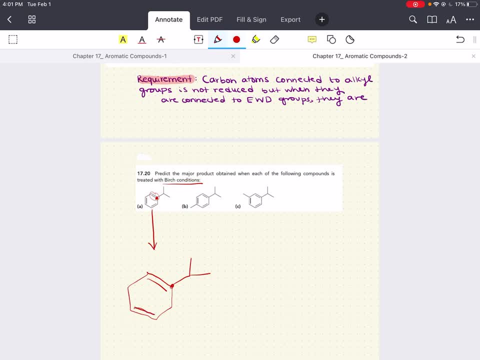 so if we know that this carbon isn't reduced and we have our double bond here, we know that the second double bond from Birch reduction forms here. All right, let's do B as well. All right, we have two alkyl groups here. All right, those carbons are not going to be reduced. So when we 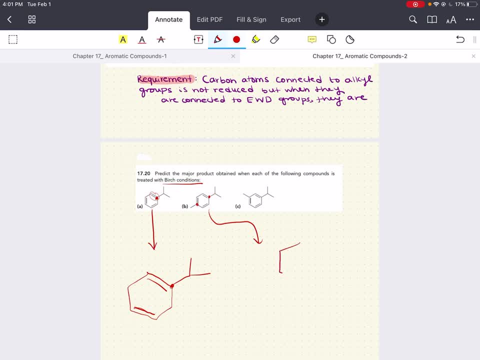 draw our Birch product. we have to keep that in mind, All right. so we're going to draw our double bond here. We have to keep that in mind. All right, we have to keep that in mind. So we have our two alkyl groups here. All right, these carbons cannot be reduced, So what we can do is 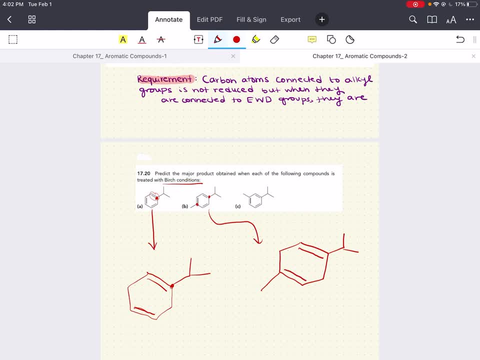 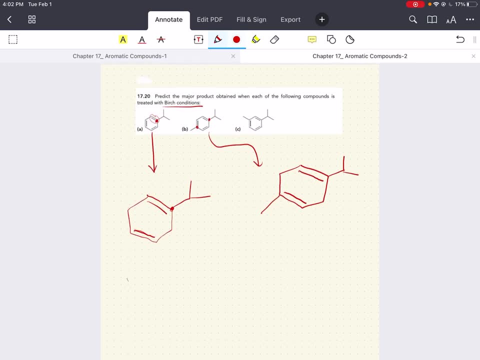 draw our double bonds like this, where they're parallel to each other. We have this again: 1,4-cyclohexadiene configuration. All right. now for C. again we have these two carbons that have alkyl groups. Those carbons cannot be reduced right because our alkyl groups are electron. 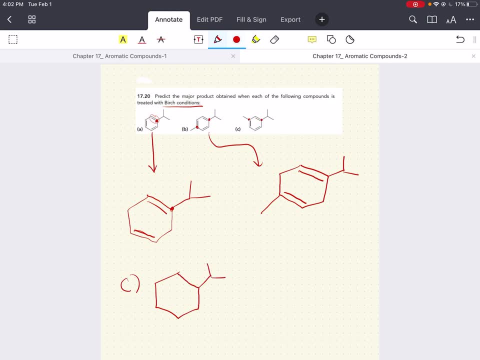 donating. We draw this. All right. how are we going to draw our double bonds here? All right, we have to preserve these carbons from being reduced. So we would draw our double bonds parallel to each other in this way. See how the carbons are not reduced. Now one thing to note. right, this is the case. 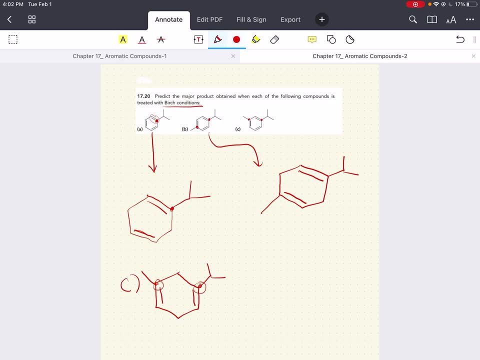 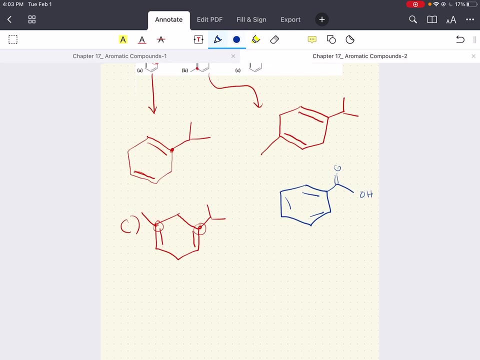 for when alkyl groups are attached, because alkyl groups are electron donating. What if you had something like this- and I'm going to do it in a different color- What if you had this as your starting material? All right, and you had, say, a carbonyl group, which is electron withdrawing, All right, when you 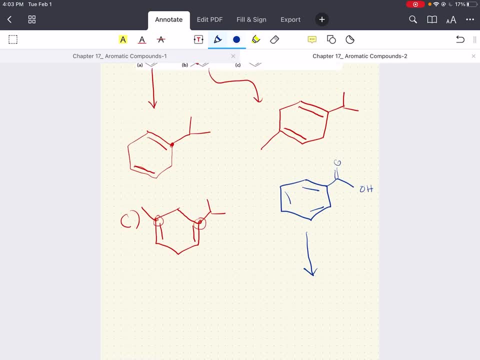 do. when you treat this with Birch conditions, your product all right. and you're trying to draw your product, this carbon is going to get reduced, All right. so that means you're no longer going to have a double bond to that carbon. So whenever you draw the product of this, you would draw the 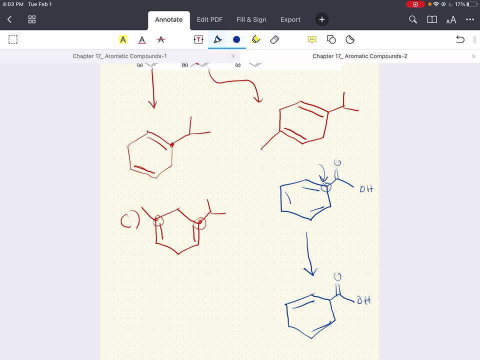 double bonds away from the electron withdrawing groups, like so. So that's how you're going to draw your product. So that's a really important point to keep in mind. All right, whenever that carbon atom connected to the. whenever there's a carbon atom connected to your alkyl group, all right. 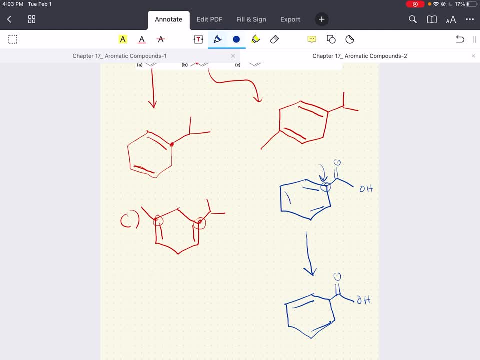 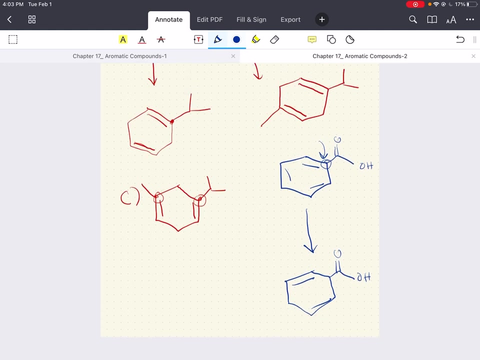 that carbon is not reduced because it's electron donating. But if you have a carbon atom connected, to say a carbonyl, which is electron withdrawing, that carbon is indeed reduced when treated with Birch conditions. So keep that in mind. I hope this was helpful. This is the last thing we had. 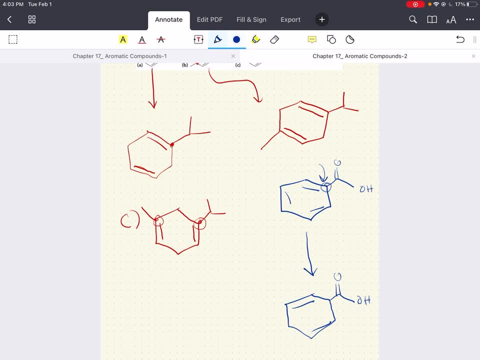 to cover. Let me know if you have any questions in the comments And I'll see you in the next video. Other than that, happy studying and good luck.